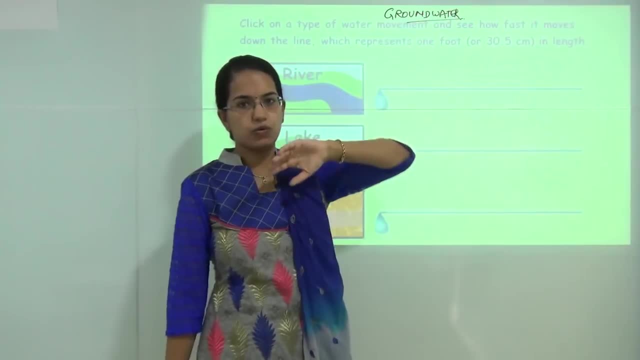 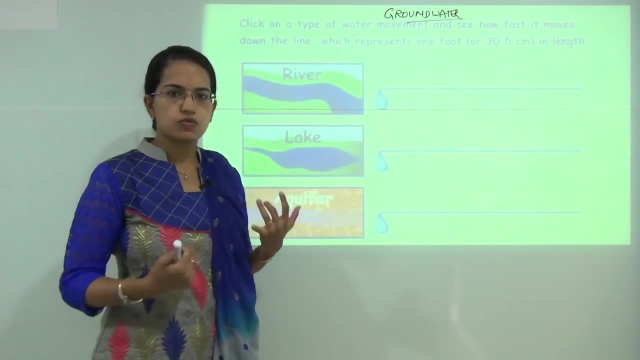 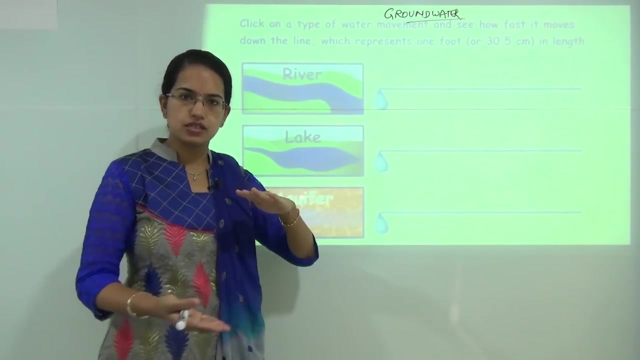 Welcome. In this session we would be talking about the concept of groundwater. If I want to classify water, I can say there is a water that runs on the surface, which is the surface water, and there is another water which moves below the surface level, that's within the 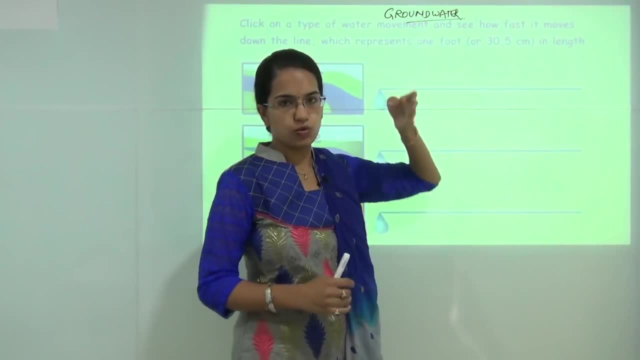 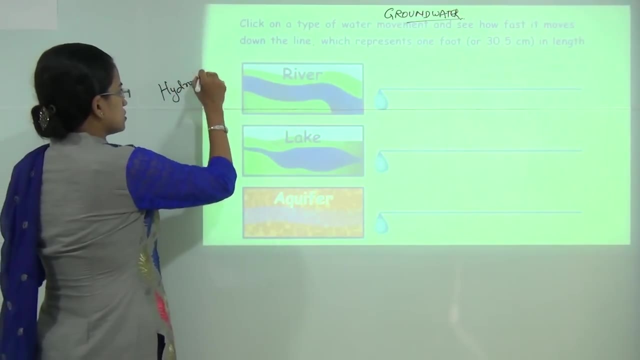 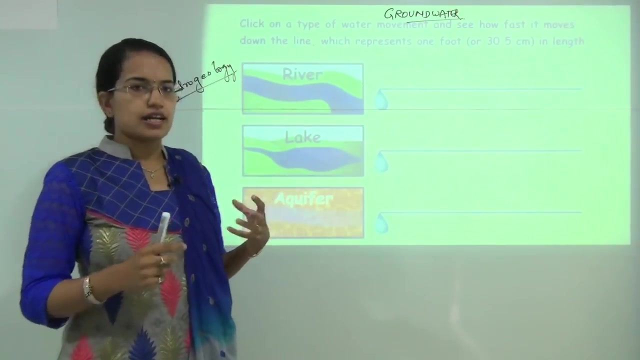 rocks, So that water would be known as groundwater. The branch under which we study groundwater is known as hydrogeology. So today we would be understanding some of the very basic fundamentals of hydrogeology. Now, before we start, let's work out a very simple example, or a very simple. 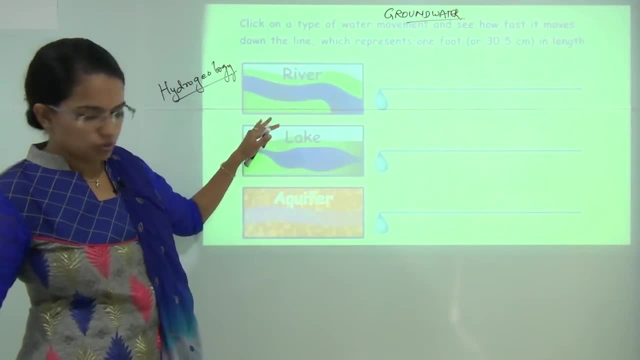 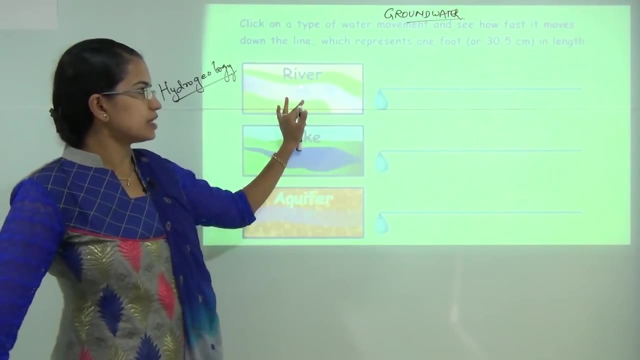 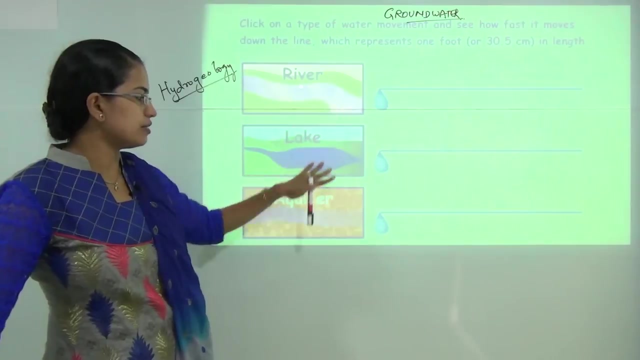 demonstration. So I have three sets here. One is river, one is lake and another is aquifer. So if I click the river here, this is from the Curtsey Michigan Technology University University. So you have this demonstration which would help you understand the rate of. 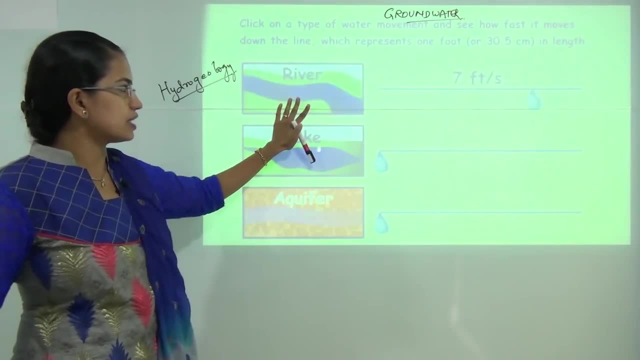 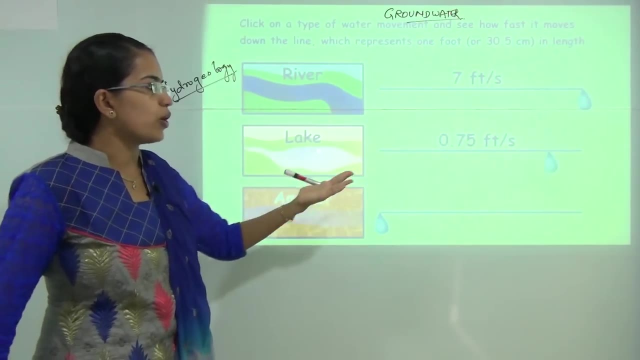 movement of the groundwater. So if I click on the river here, you can see the movement is pretty fast. It says around 7 feet per second. In case of lakes, it's 0.75 feet per second. However, let's see when it comes to underground reservoirs, When it comes to 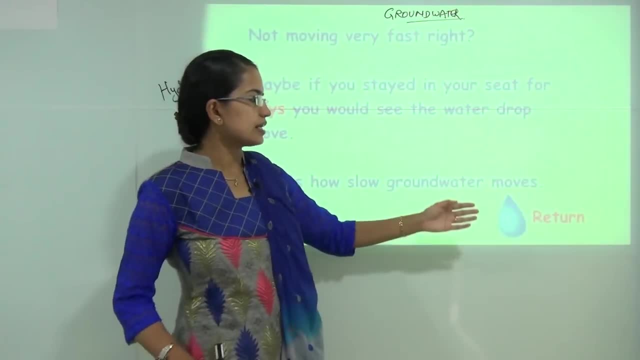 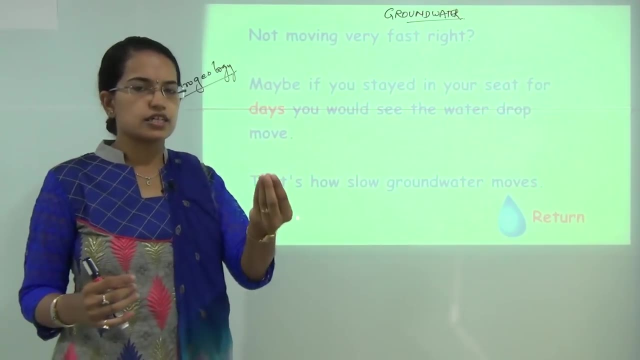 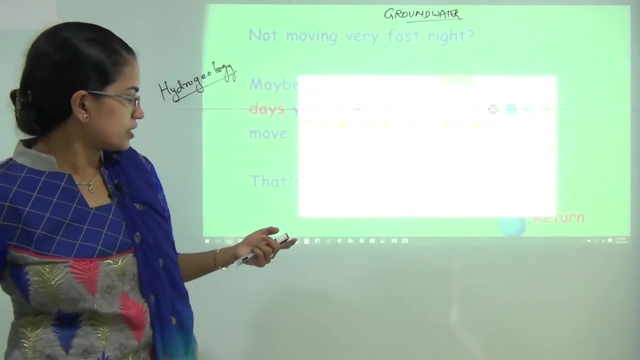 underground water. you can say the rate is 0.33 feet per day. That means if you are in the river, you are sitting there for the whole day. you might not see a drop falling down. So that is the speed at which the groundwater moves. However, it's important to understand. 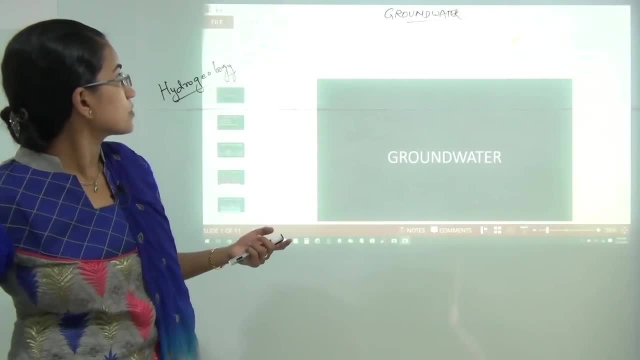 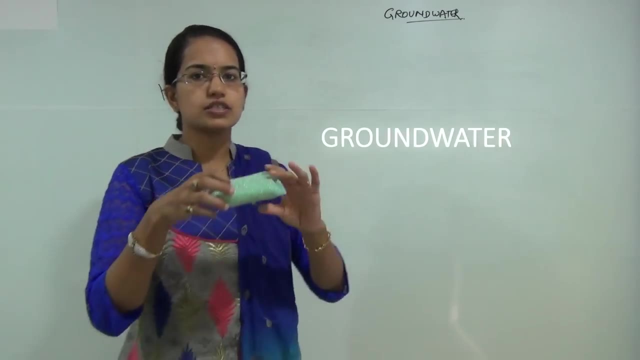 that it's not just the movement that we would be focusing today. We will try to understand the various fundamentals related to groundwater. To demonstrate this, I have a sponge here. Consider this to be a part of underground topography. Now, these suppose these to be. 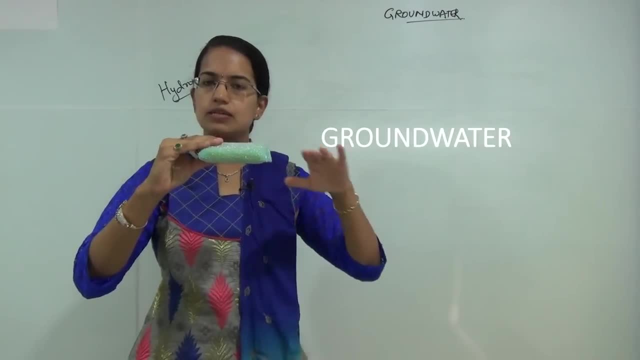 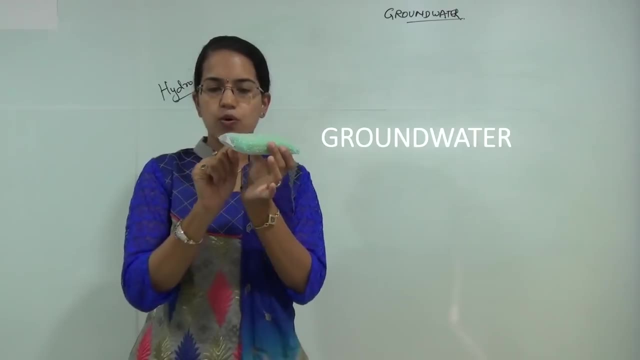 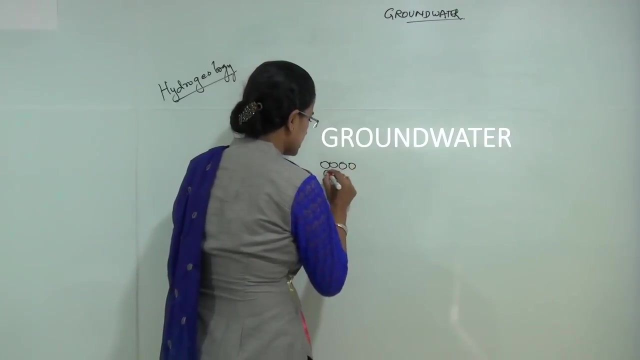 a sequence. This is a section of rocks which are present below the surface of the earth. Now what would happen here? This sponge is porous in nature. Porous means there are small holes, or I could say the arrangement of the particles are in such a fashion that there is spaces between. 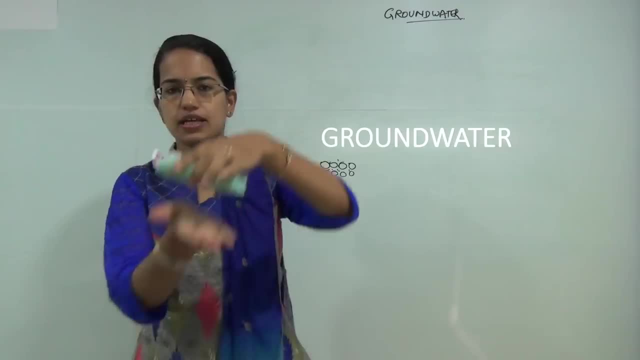 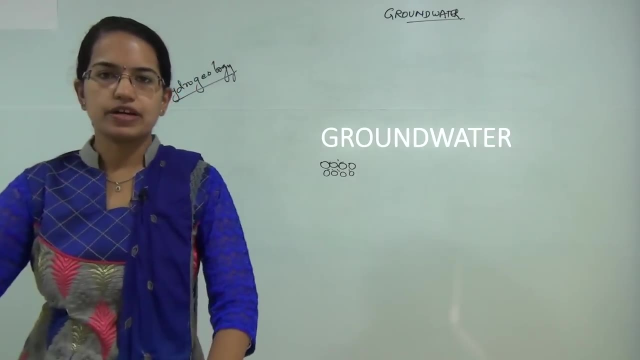 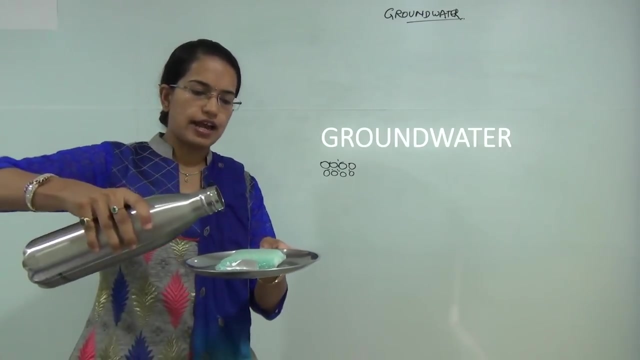 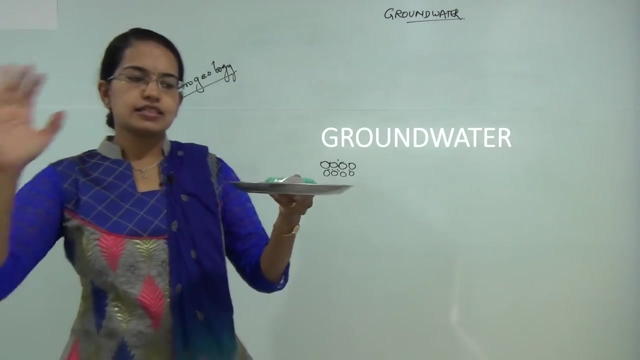 these particles and those spaces can be compressed. So if I want to compress this, I can compress it and it would reduce in thickness. However, what I am trying to explain today is how underground water moves. So I have a plate here and I am pouring some water on this piece. Now let's try to understand when. 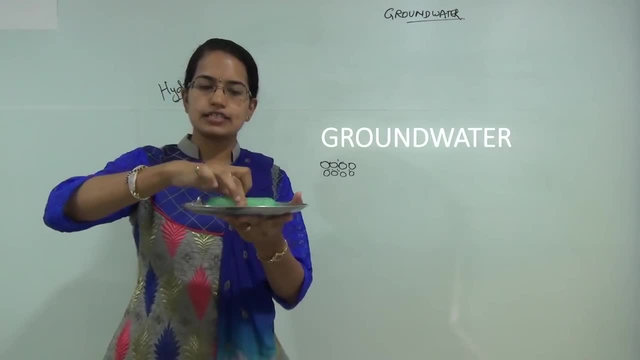 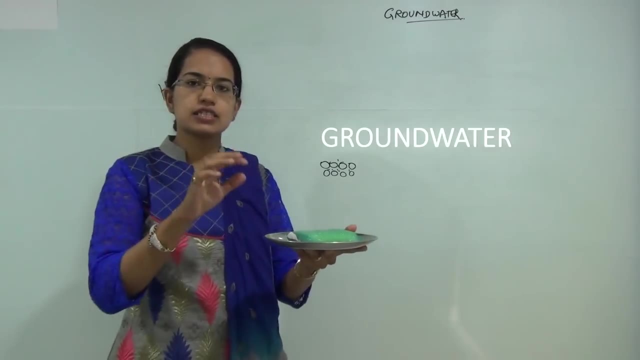 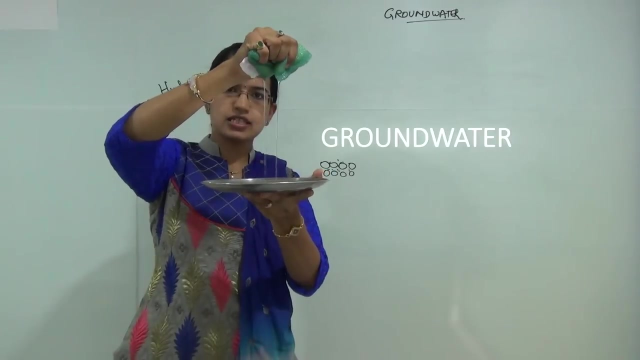 this system is in equilibrium. you have the water that this sponge has absorbed. Now, what would happen in the case that there is an aquifer that is being pumped? So if I am pumping an aquifer, that means there is water that is coming out Similarly, from the underground. 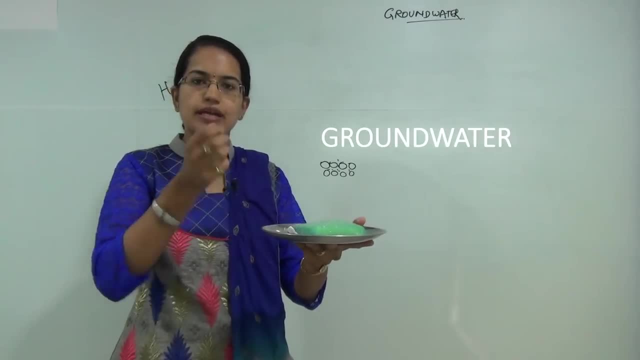 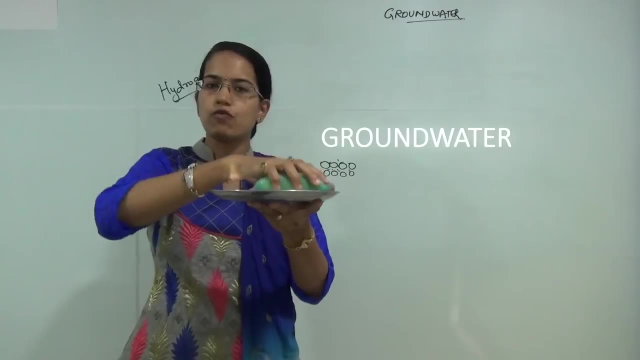 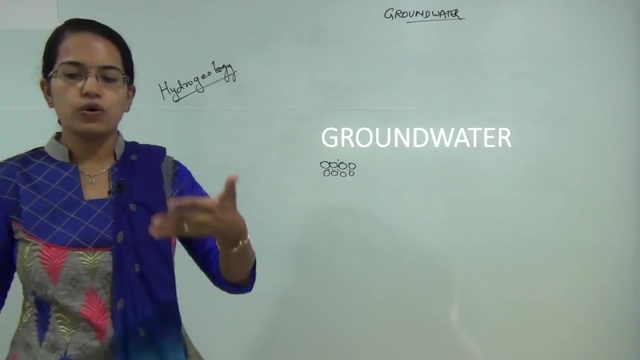 systems, water can come out only by means of pumping. So you have definitely a huge lot of water that is present here and once you pump it you would have water that would come out onto the higher elevations. So that is how the principle of aquifers is understood. 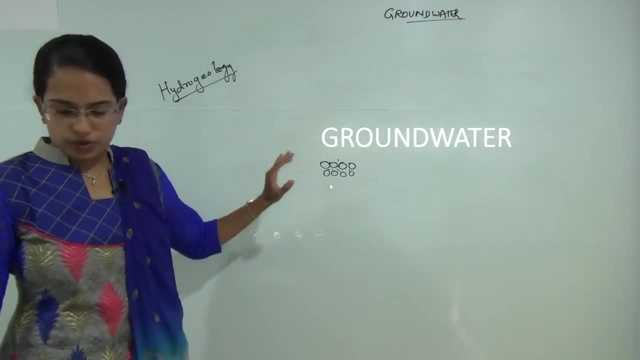 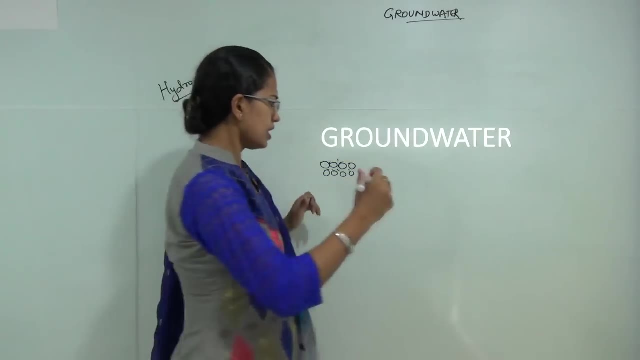 and how the water table is maintained. So that's it, Thank you. 1. So if I try to understand the groundwater, I can say the water that is present in the surface below the earth. However, within the groundwater there can be various types. 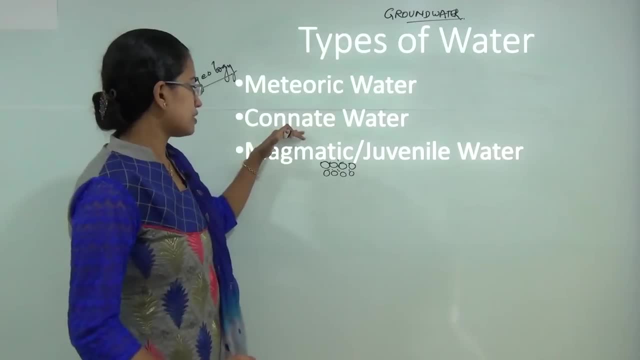 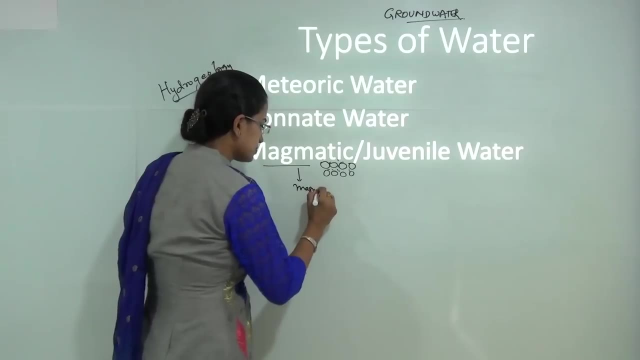 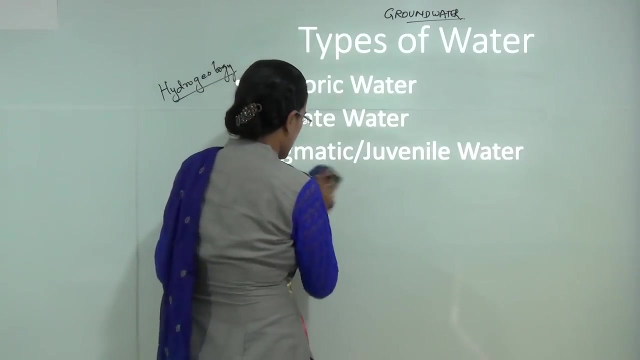 of water. The first is the meteoric water, conate water and the magmatic water. The magmatic water, as the name suggests, is derived from the magma, So it's mainly found in the igneous rocks. 2- The magma rises and as the magma rises you have water that rises to the surface. Then 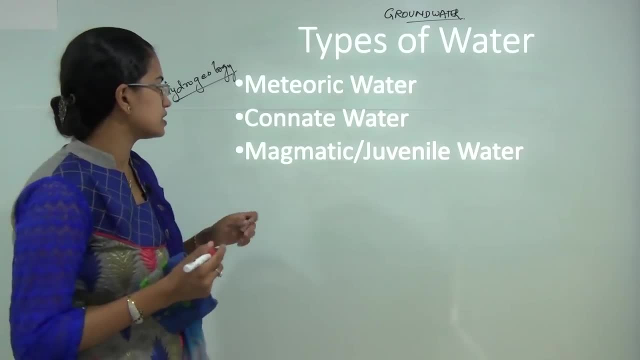 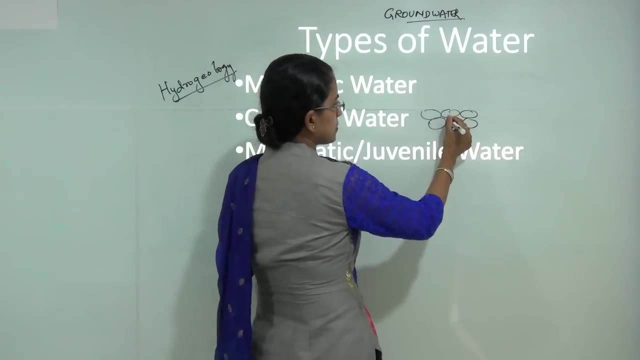 you have the conate water. Conate water is the water trapped within the rock mass. So, if you have, like the case of sponge we discussed, you have the rocks and the water that is present within the rocks would be known as the conate water, And then you have the meteoric water. 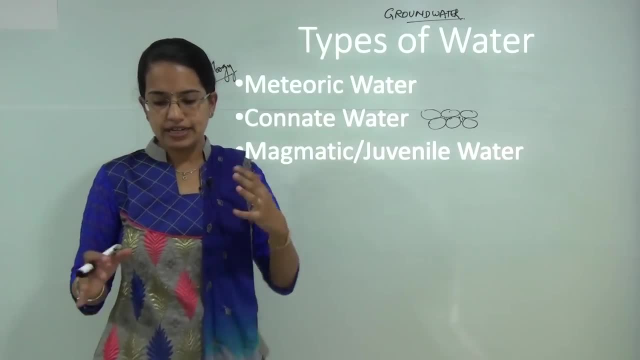 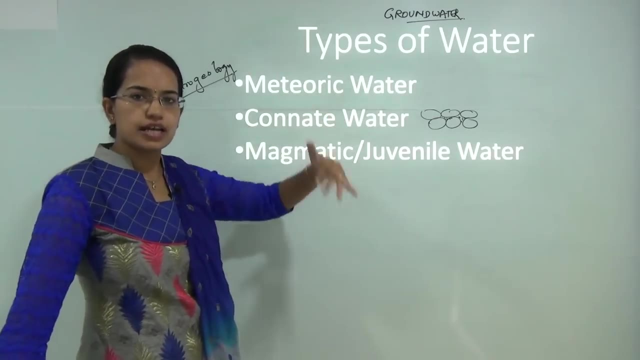 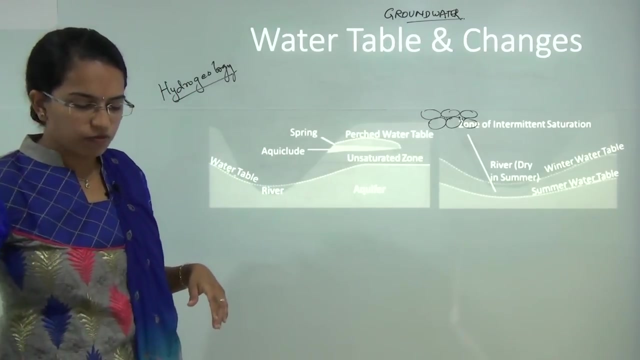 Meteoric water is the most long standing water that is present and it is the main source of aquifer recharge. 3, And this water is mainly generated from the rainfall or the atmospheric precipitation. Now, to understand the zones, we must understand the concept of water table. When I say water, 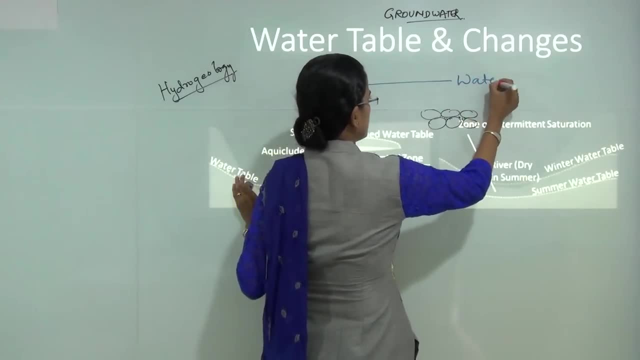 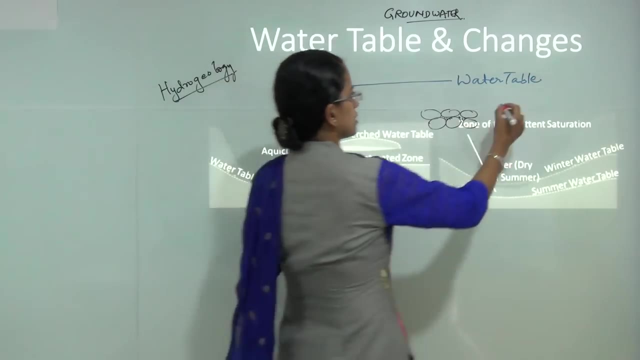 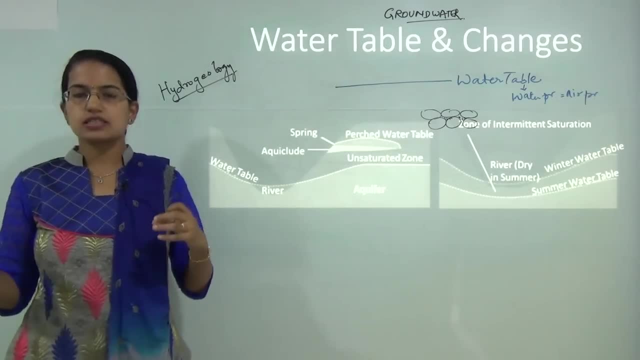 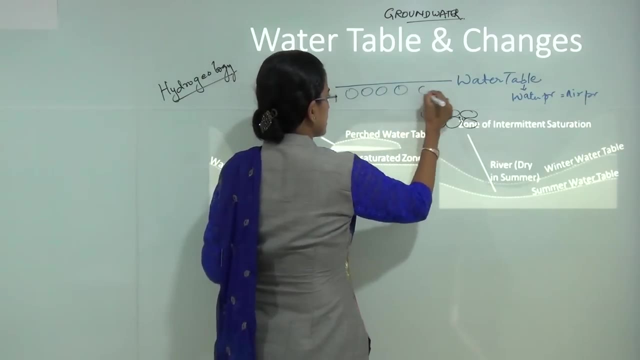 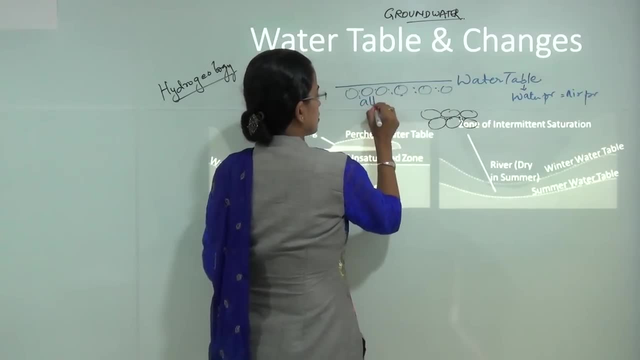 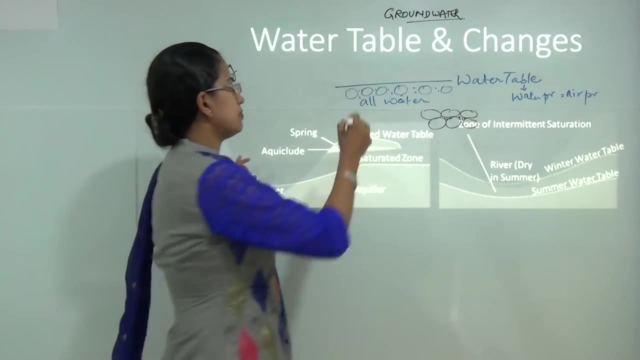 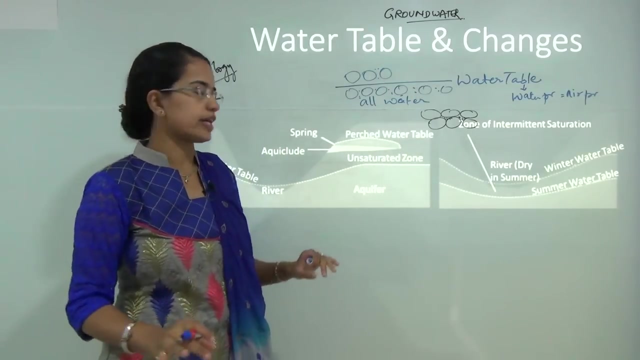 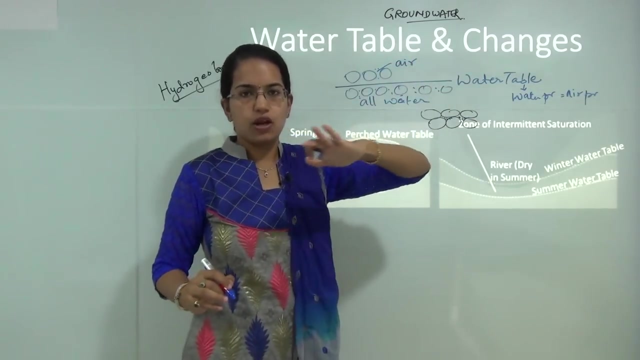 are occupied with water, So there is all water. I could say that is below this water table. However, above this water table, when there is rock and there are pores, it need not have presence of absolute water. 4 have intermittent air in it. however, below the zone of water table or below the water, 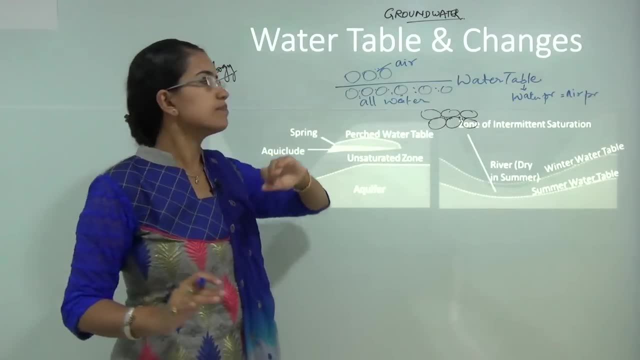 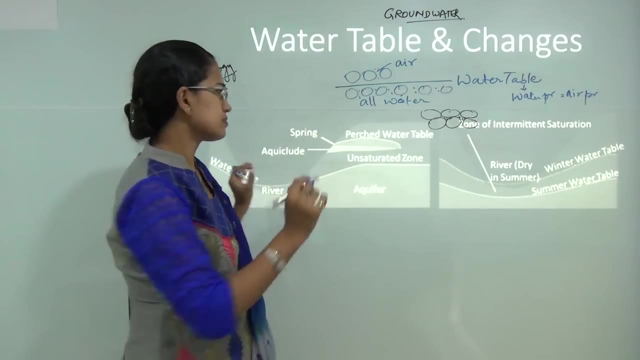 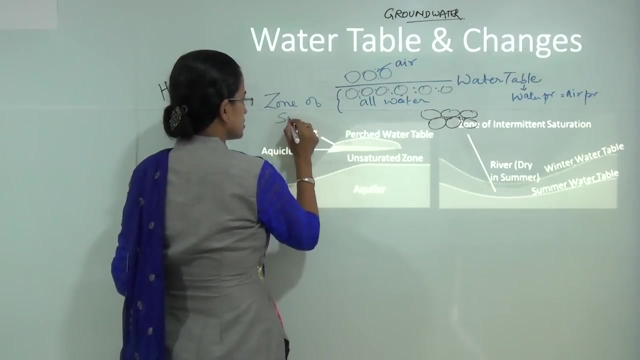 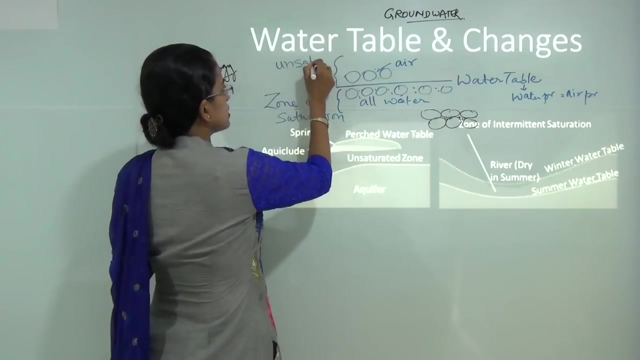 table, all the pores would be filled with water. but above the water table you can have some water, but it would be mostly air. therefore, the zone below the water table is known as zone of saturation and zone above the water table is known as zone of unsaturation, since 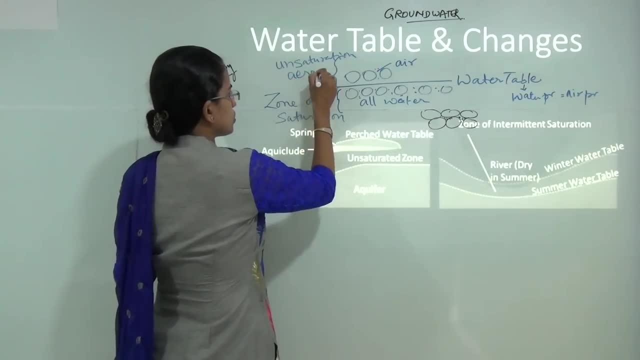 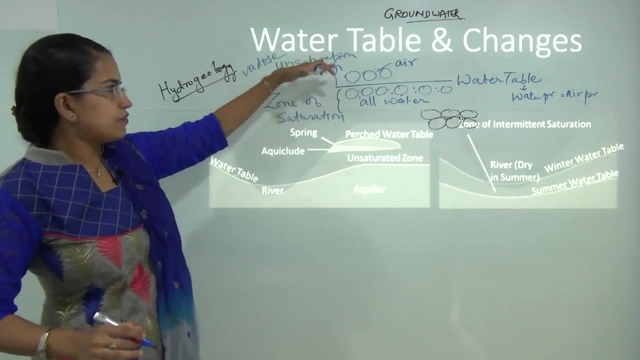 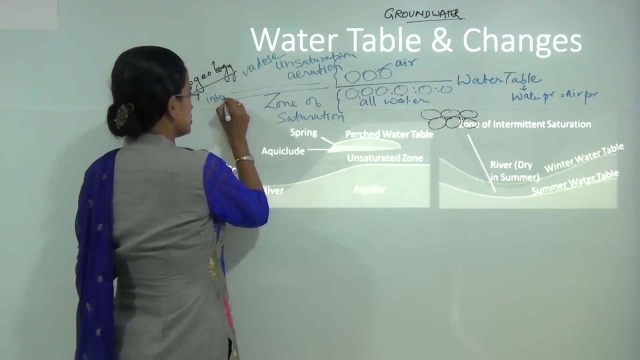 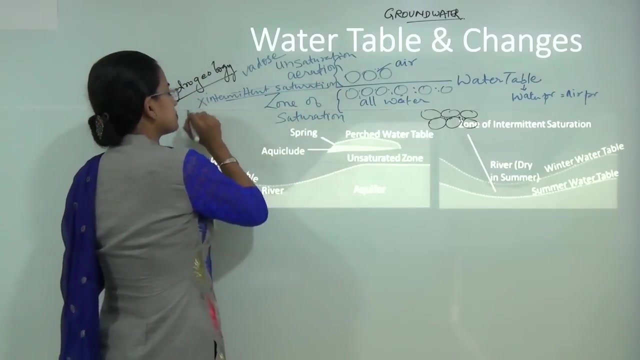 you have air that is present here. we also call it zone of aeration and it is also known as weathers zone. between the zone of unsaturation and zone of saturation, sometimes there is a intermittent saturation zone that is present And this intermittent saturation zone, I can say, is not 100 percent saturated with water. 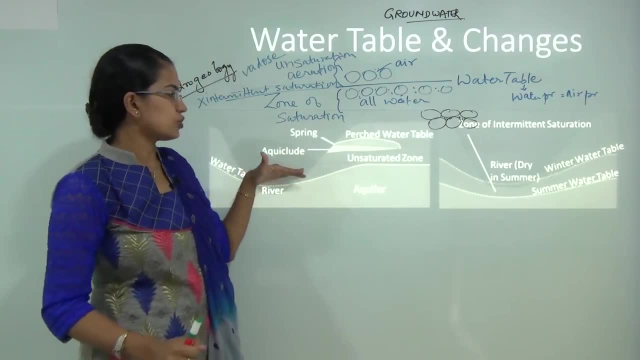 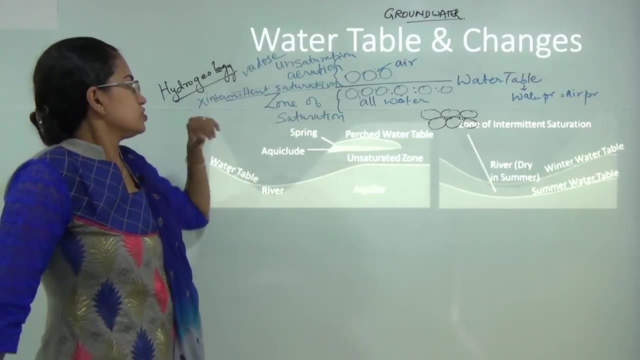 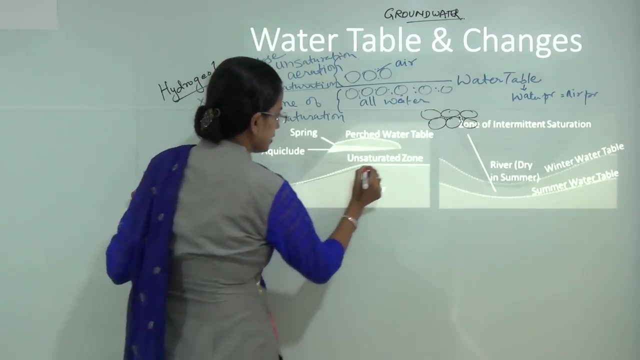 it is intermittent in nature. and finally is the zone of pharyatic. that is, the zone where the- I could say- groundwater is at the atmospheric pressure. So these are the four zones that we try to understand now in this diagram. you can see the water table here. above the water table you have saturated water and below that you. 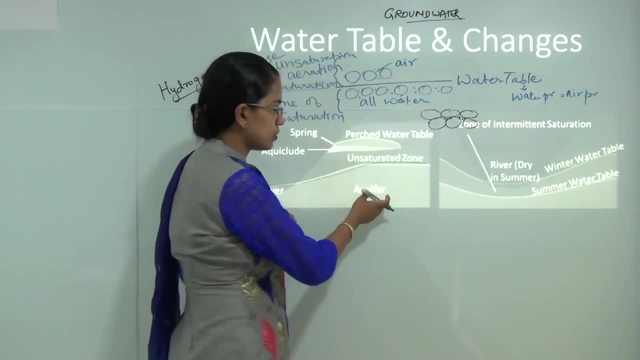 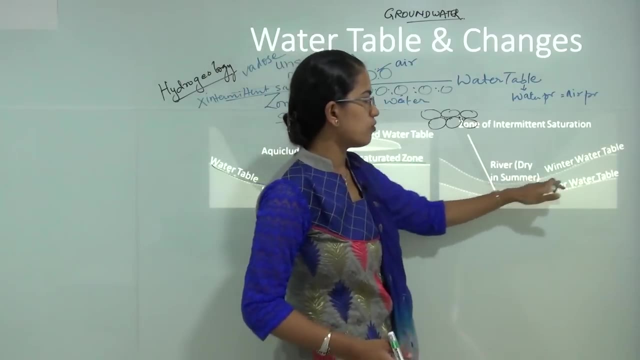 have unsaturated water. have the sorry. above the water table, you have unsaturated water, and below that you have the aquifer. however, this water table keeps on changing. in the winter months, the water table is at a higher elevation. however, during summer months, water gets pulled out. it gets. 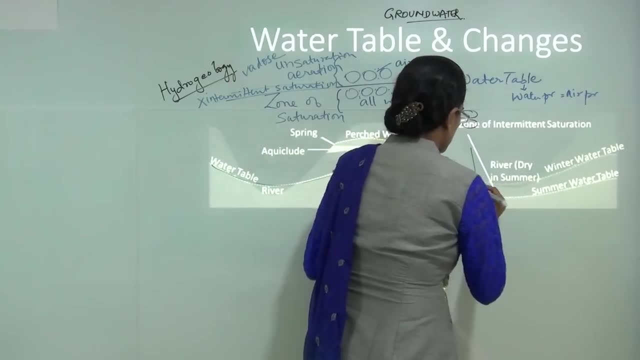 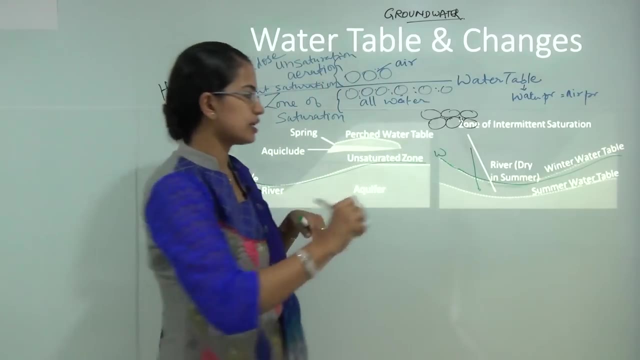 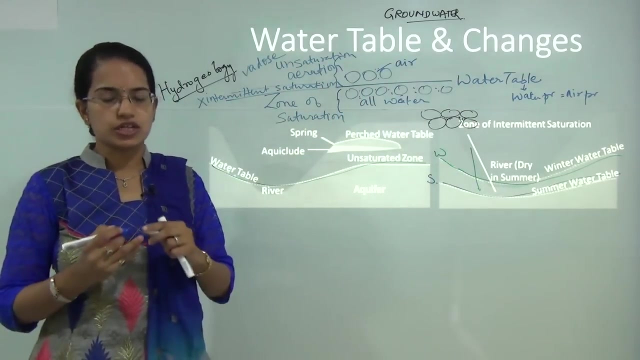 dried and the water table moves down. so you can see the changes in the water table. so this upper line shows the winter water table, the water table line during the winters and this shows the water table during the summers. so in summers generally the water table or the level of water drops down. 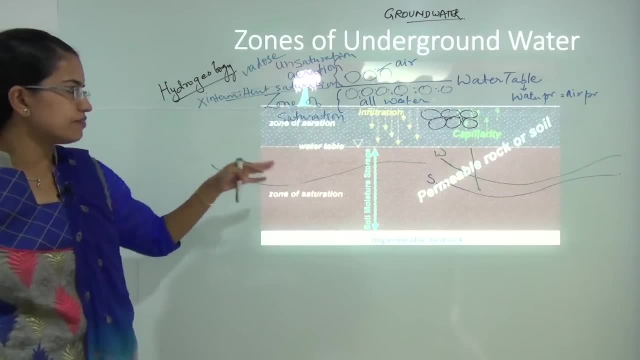 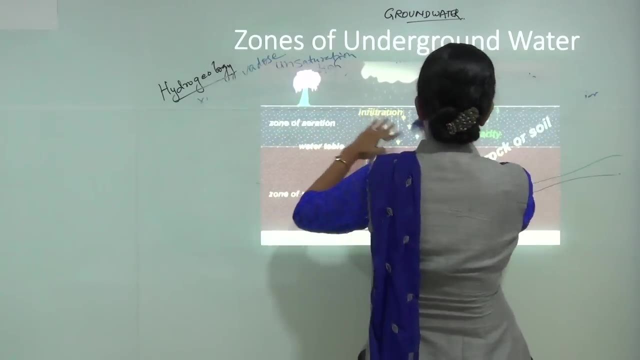 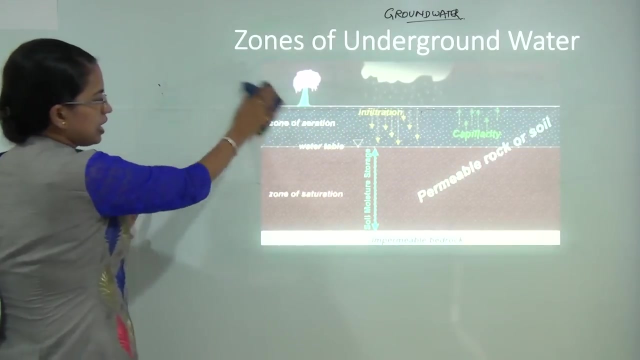 Now, in this diagram, you can understand how infiltration takes place and once the infiltration is taking place, the region above the water table, which is zone of variation- you have the infiltration and the capillary action that is predominant, however, towards the zone of saturation. It is the zone of variation. 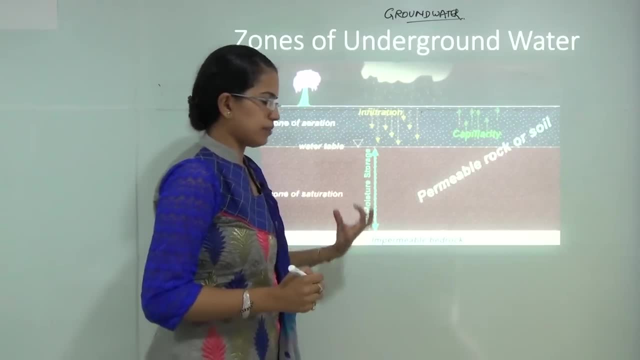 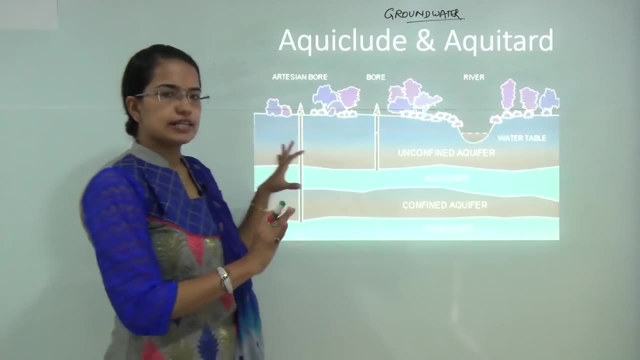 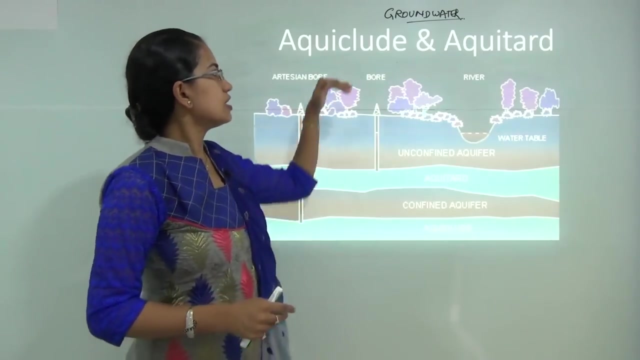 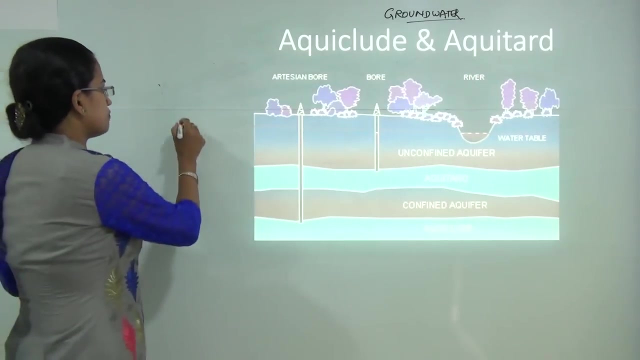 It is mainly the water is stored as soil moisture. now there are few terminologies that we must understand to comprehend this topic in more detail. the three terminologies that we would be focusing today is aquifer, aquiclude and aquitard. Now we must first understand the difference between the three terms. so the first is aquifer. 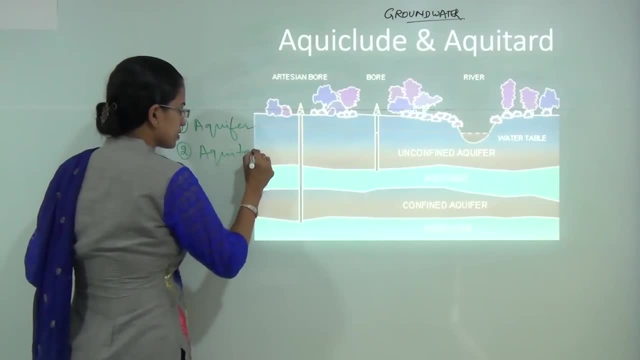 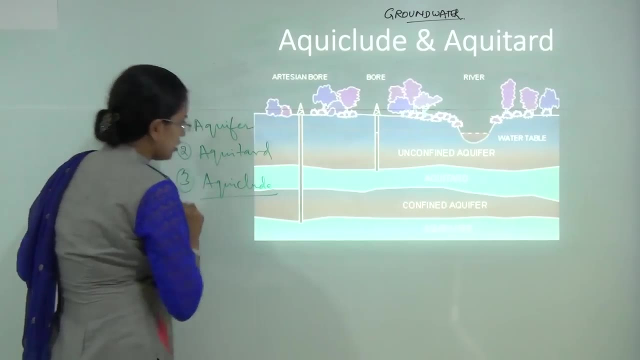 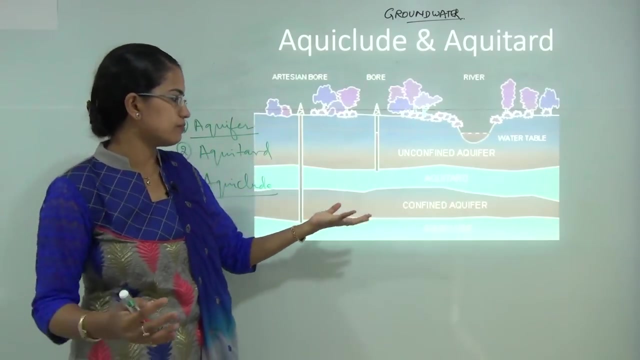 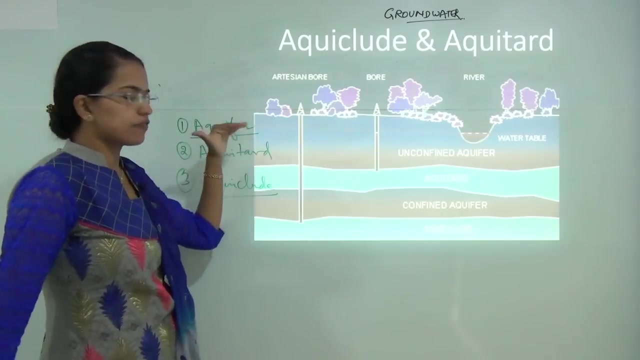 the second is aquitard and the third is aquiclude. let us first start with aquifer. A QFER is a region, or I could say it is a body of large permeable material that has enough water it can hold and it lies mainly in the saturated region. 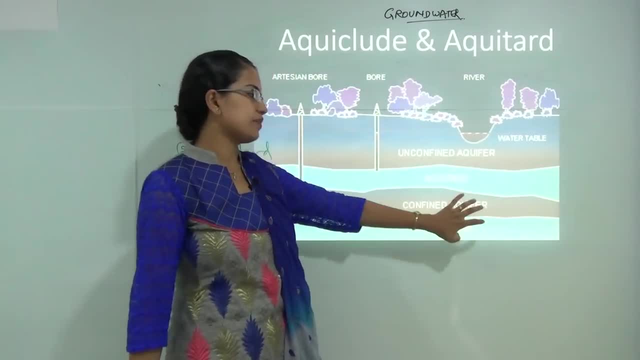 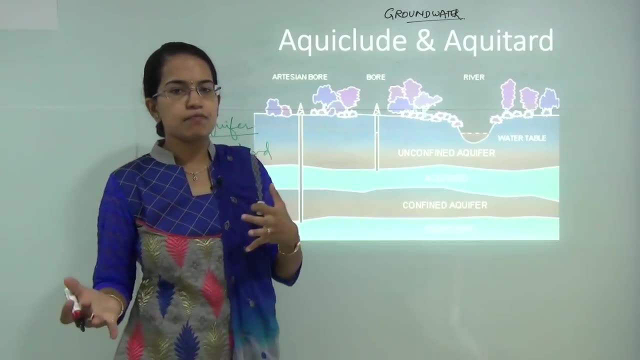 This aquifer can further be classified as confined aquifers and unconfined aquifers. unconfined aquifers, confined aquifers- are those which are confined between two impermeable rocks. now, when I say permeable and impermeable, permeable means through which water can pass. 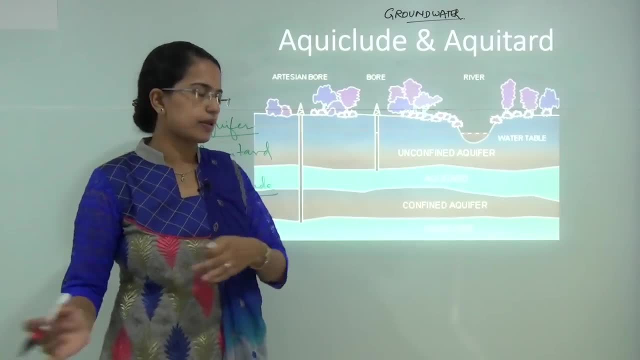 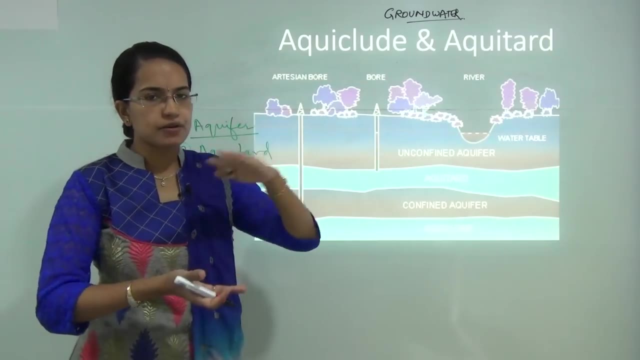 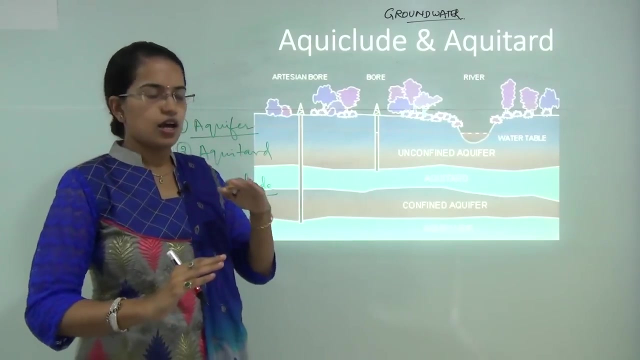 or which has kind of permeability. we will be talking about permeability further in this class. so you have confined aquifers which lie between two impermeable layers. so those two impermeable layers do not allow flow of liquid from those sections. so these confined 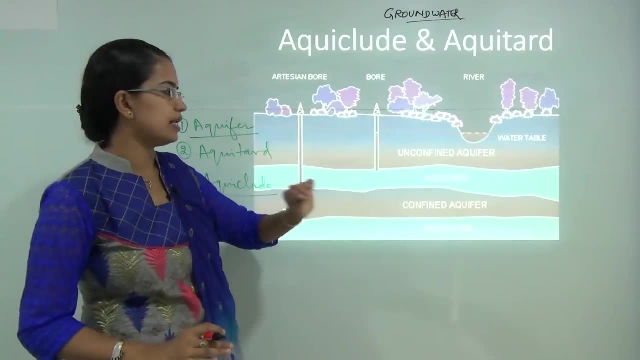 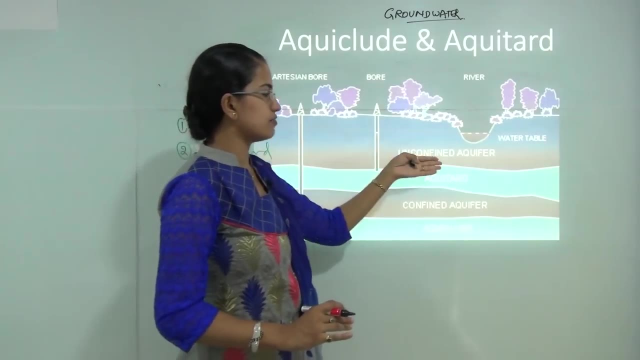 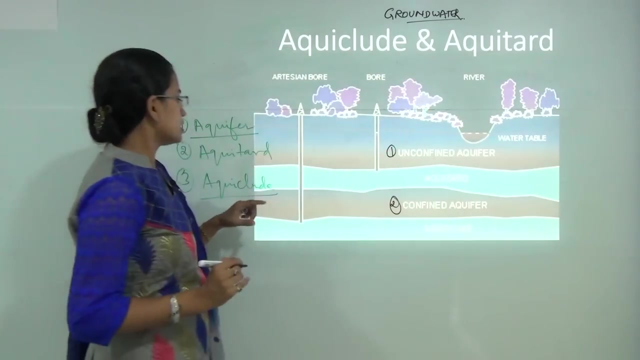 aquifers are confined within two impermeable layers. however, unconfined aquifer is usually exposed to the surface, so one part of the unconfined aquifer would definitely be exposed to the surface. so you have unconfined and confined aquifers now. next is aquitard. aquitard. 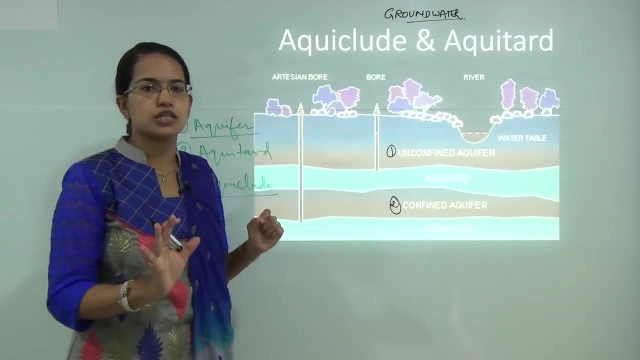 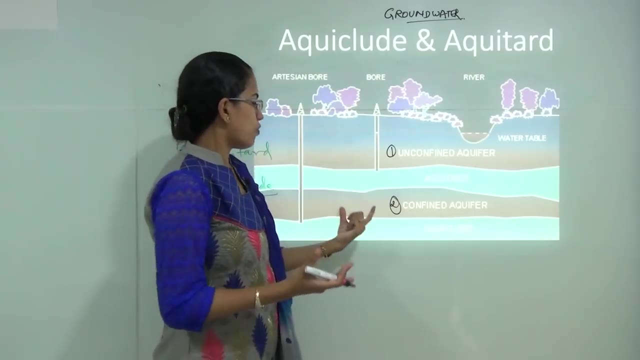 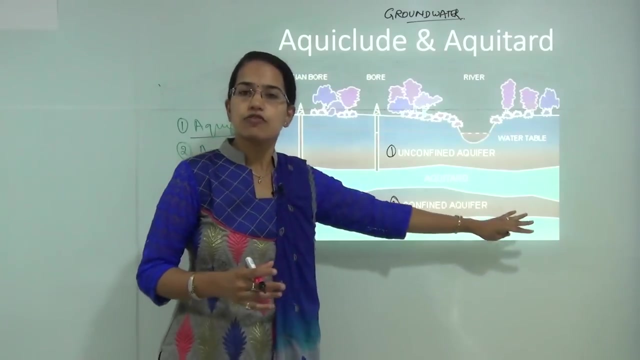 I could say. say in simple terms: it is opposite to what is aquifer. in aquifer you have the water that is available. the water in the aquifer region would have good porosity and permeability in those region because the water is flowing in that region. however, aquitard can be made. 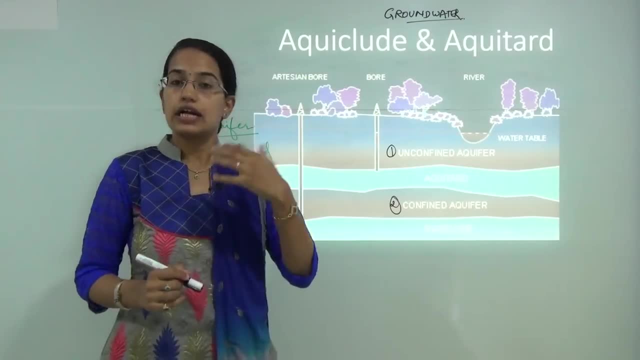 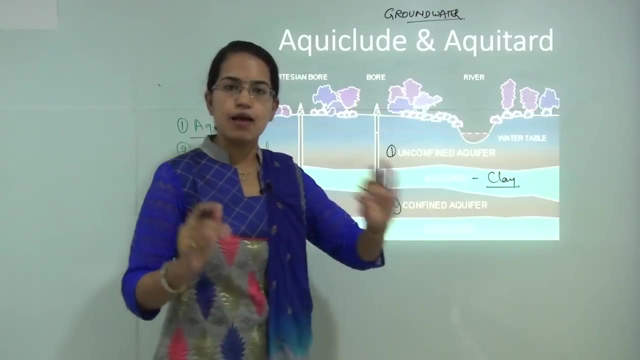 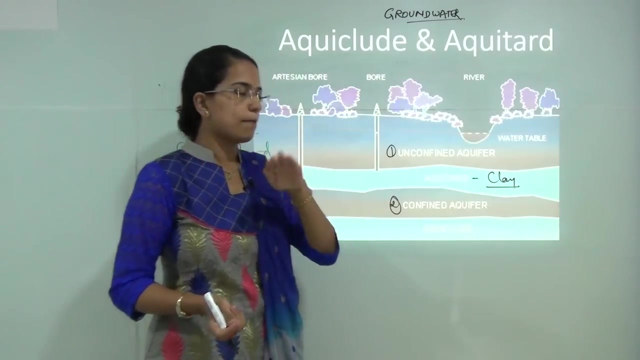 up of any substance. say, for example, I could say clay is one of a very good examples of aquitard. now what would happen? this clay has ample porosity. porosity means it has ample pores within it so it can hold water, but this layer of clay wont allow movement of water. 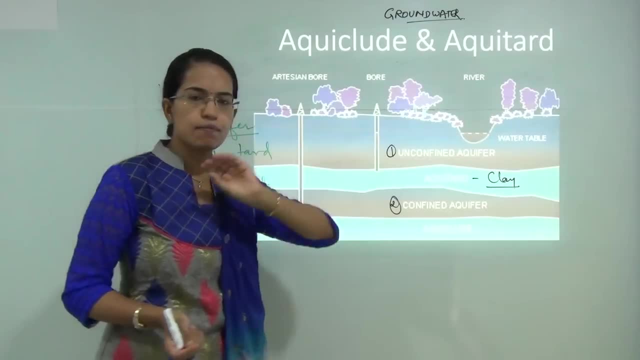 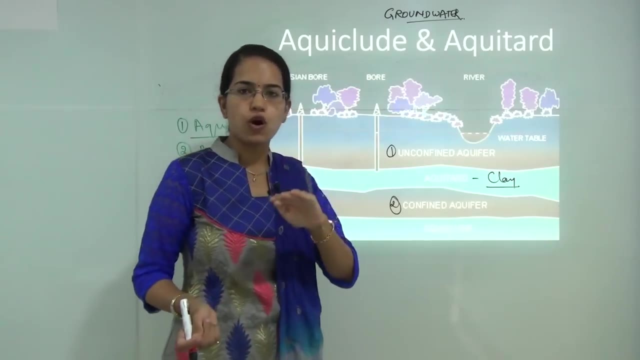 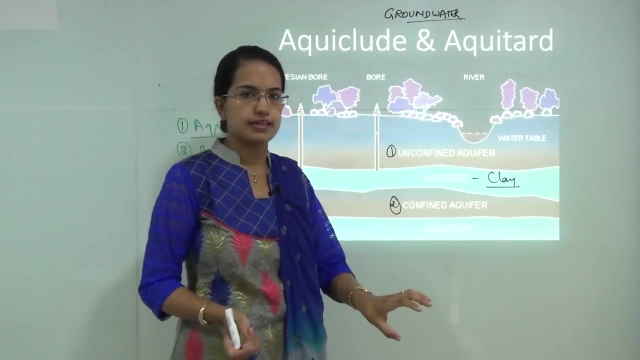 from one region to another. so aquitards, in simple terms, act as a barrier between two aquifers. they do not allow movement of water from one aquifer to another. so they are different from one region to another to another aquifer. however, note that they can hold water by themselves. it's not that. 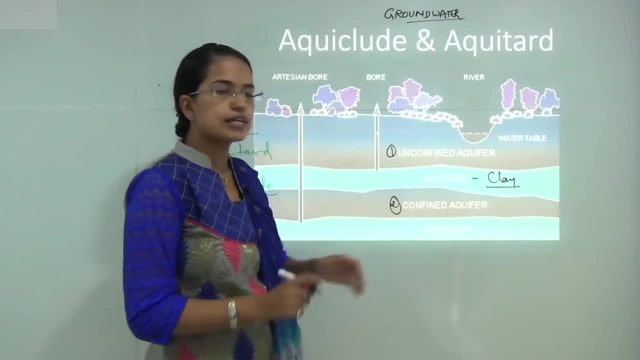 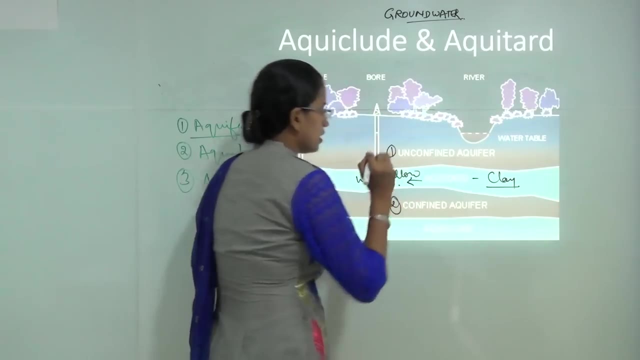 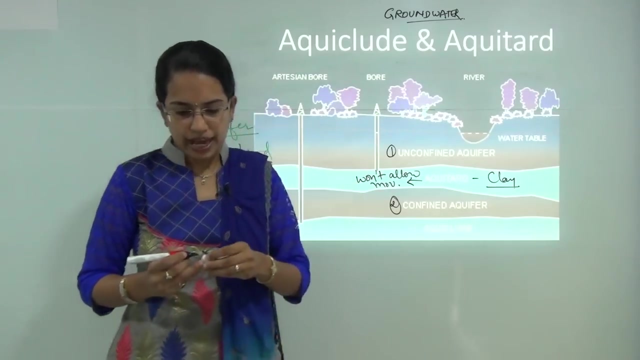 they cannot hold water. they can hold water, but they won't allow movement of water. so aquifer- sorry equator- is the region which won't allow movement of water. now, what is an aquiclude? aquiclude is a impermeable rock that acts as barrier, and it can. it's usually 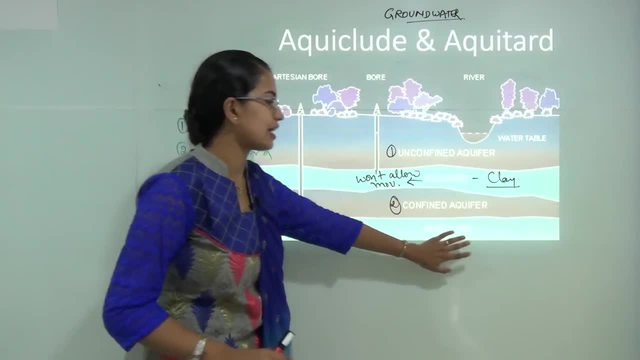 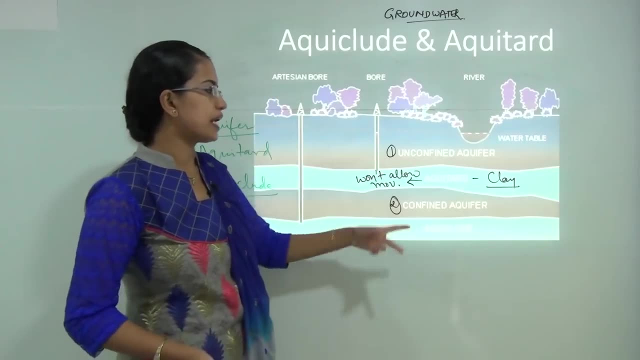 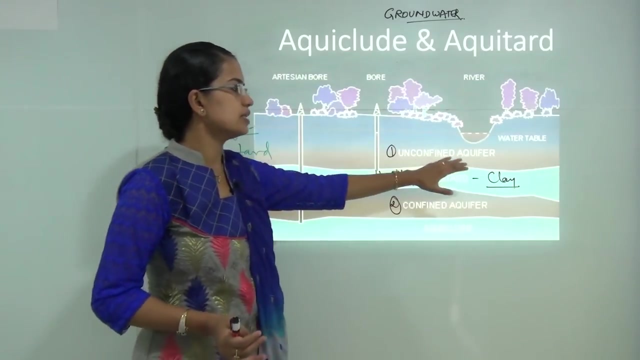 found at the lower most layer, and it's not necessary that aquiclude separates two aquifers. however, equator in general separates or distinguishes two distinct aquifer regions. so those are the three terms that are commonly discussed when we talk about more about hydrogeology. 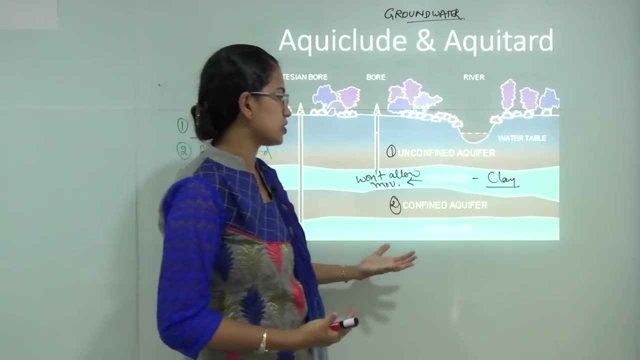 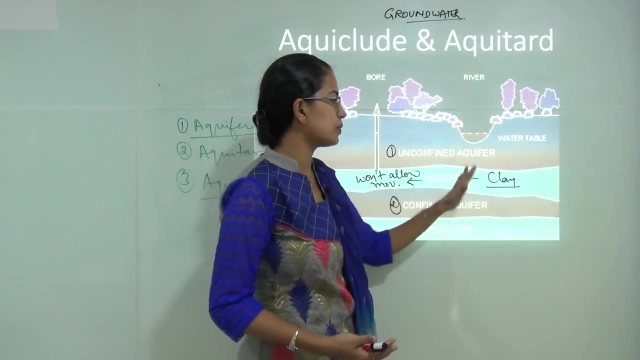 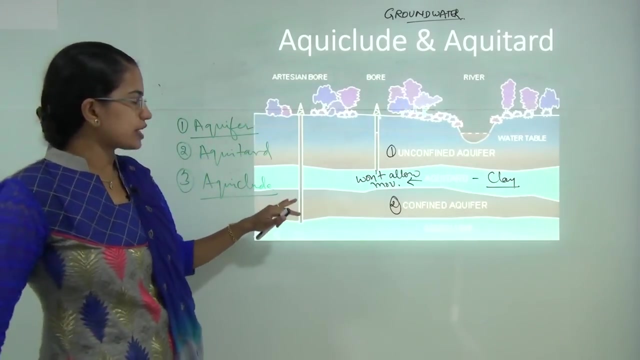 when we talk about hydrogeology, We will be discussing the more detailed concepts on hydrogeology. we will understand that these three terms are the commonly discussed terms and therefore it's very important to clarify the doubts within these terms and the concept of porosity and permeability. so this was what 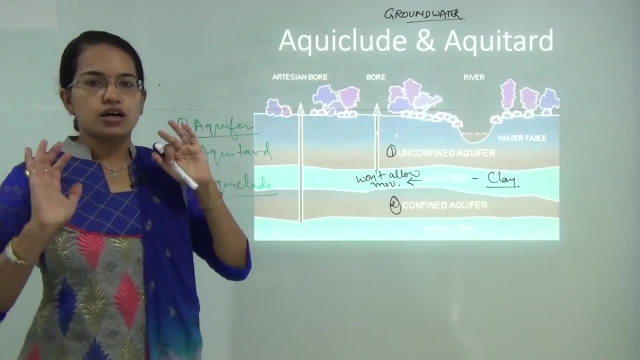 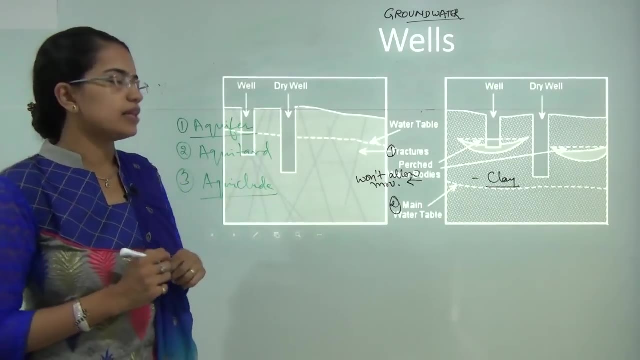 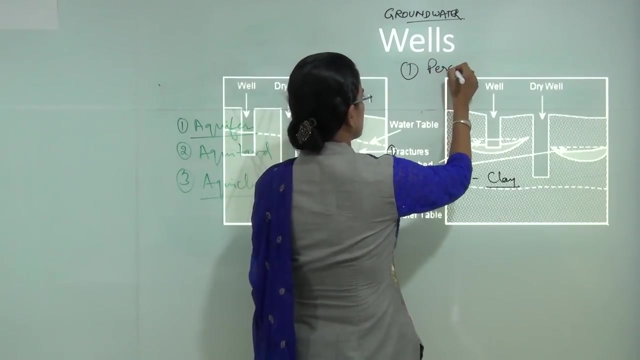 is the basis of ground water. Now, we already talked about the water table. however, when we talk about water table, there are some other items that we need to discuss. first is the perch water table, the second is the springs and third is the wells. so when there is underground water, I can say: there. 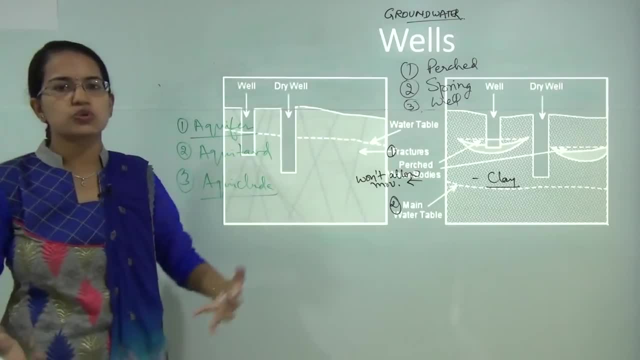 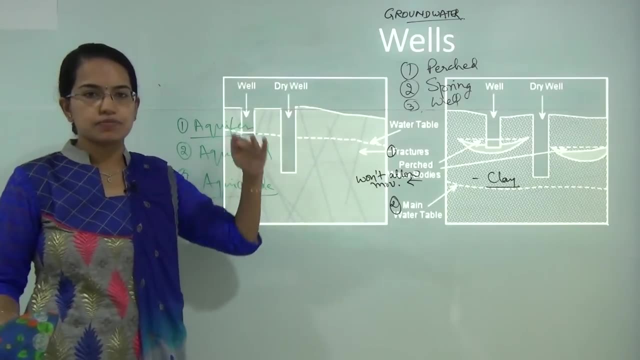 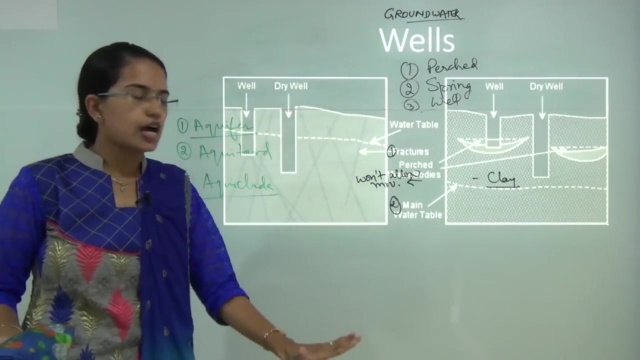 are three ways in which you can extract the water. we already talked about the water table, the concepts of water table, how the depth increases in summer. so the depth of water table would increase in summer. that means the water table level would increase and aumentol go down. so that is the basic concept of water table. now let's talk about purged water table. 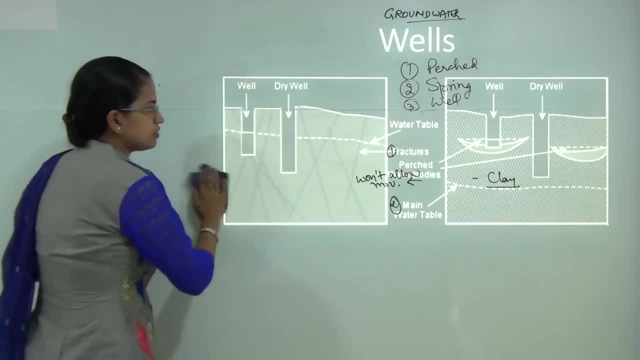 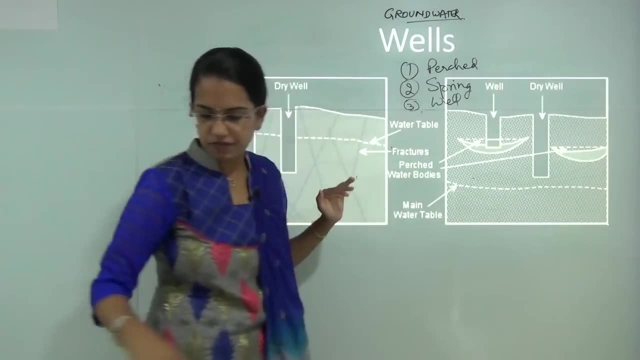 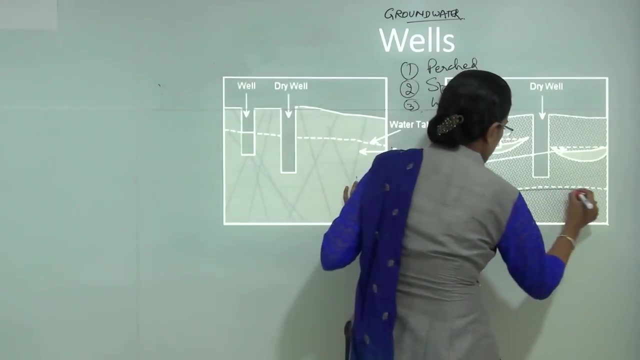 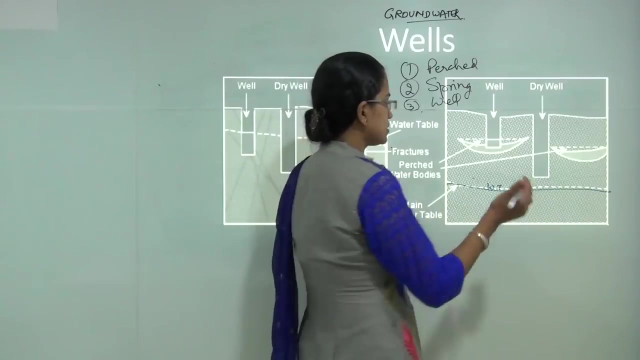 purged water table means the actual water table lies at a separate level. however, you have sections of water bodies that are filled above the main water table. so, for example, in this diagram you can see you have the main water table level that lies here. however, above the main water table level you have sections where you have water that is filled up in. 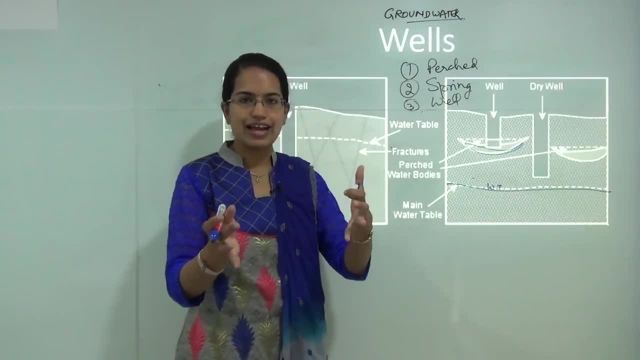 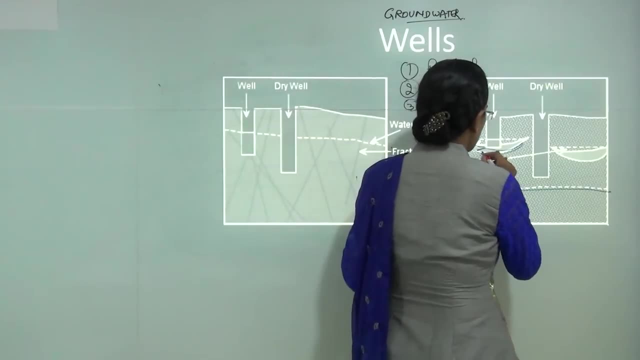 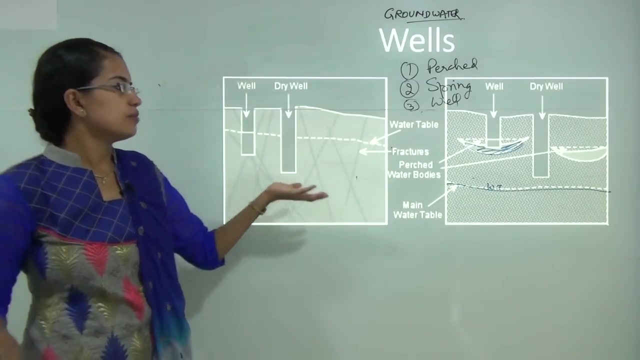 pouches, these? when I say pouches, it's not actually small pouches, they are huge extensions of. they are huge extensions basically. so you have the purged water table that is present above the main water table, and this purged water table helps to bring out water. so for 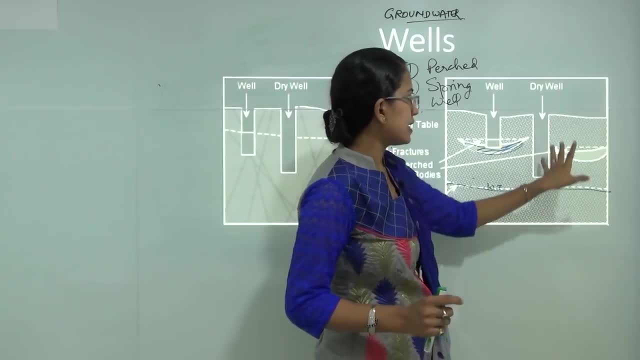 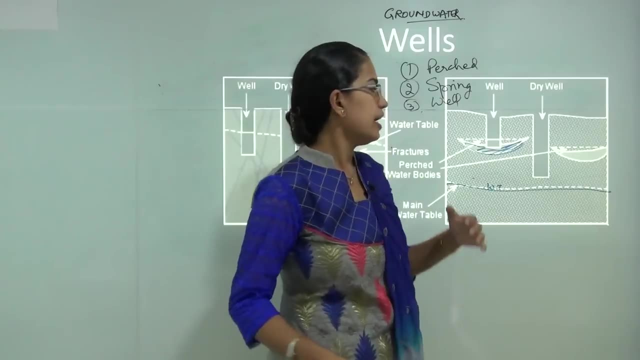 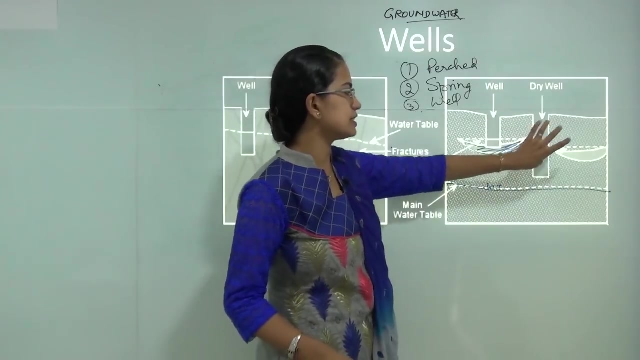 example, if I am digging well in this region, If I dig a well Well here which does not have a purged water table, even if I dig it so deep, it would remain dry. however, if there is a purged water body that is present here, even if I dig a well. 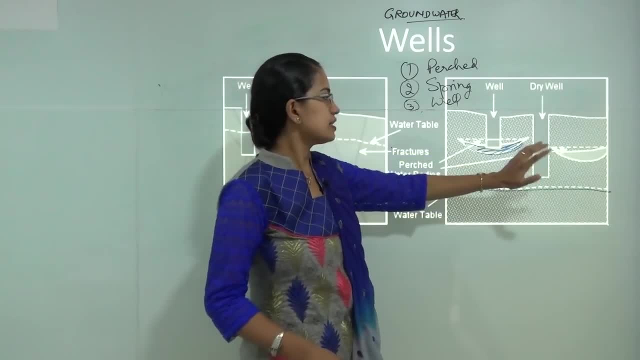 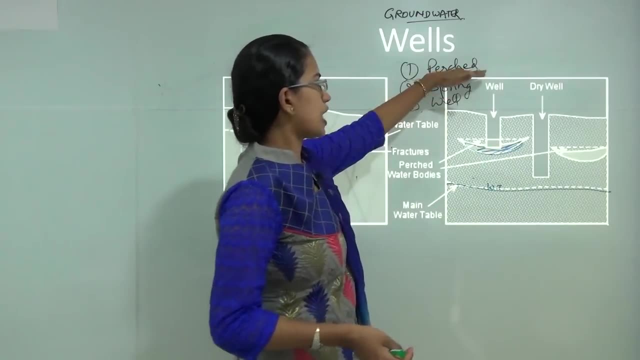 which is at a lesser depth as compared to the dry well. despite of that, this well would have ample of water. that is due to the presence of purged water table. so that is the first thing that we try to understand. under ground water reservoirs, that's the purged water table. 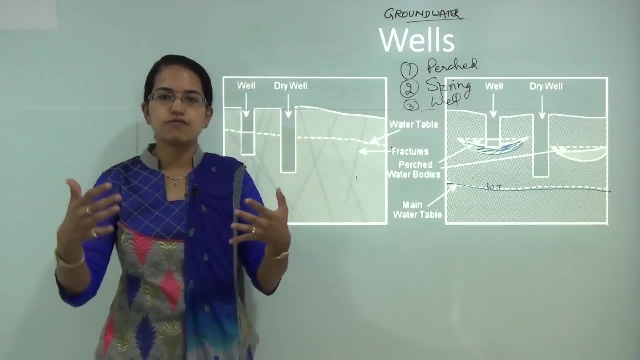 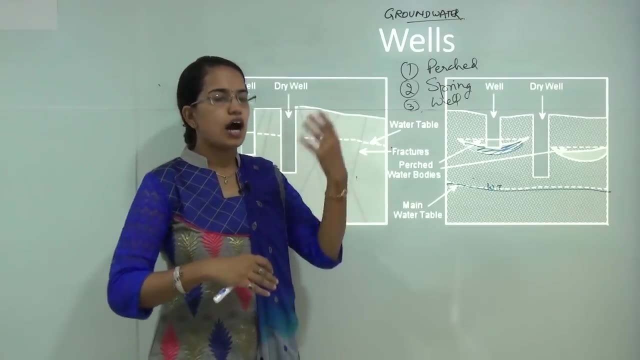 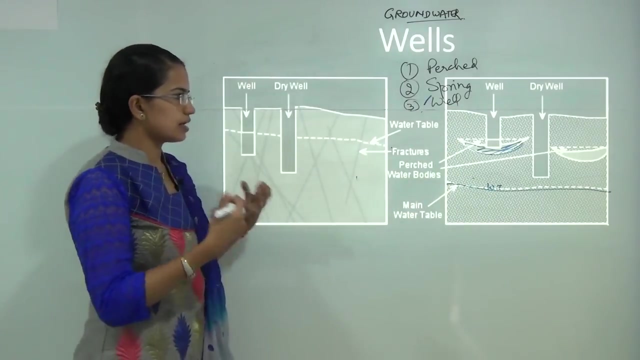 the next is spring. Spring in general is the region where water table tries to intersect at the surface, and when the water table is intersecting at the surface, there is outcome of water, so it's in the form of spring. The next is well. well is a phenomena which is dug by human beings. so you have this as 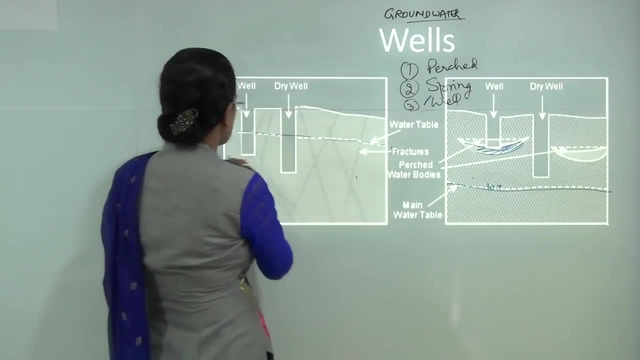 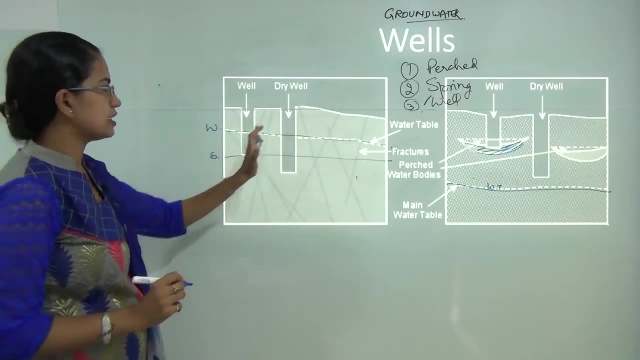 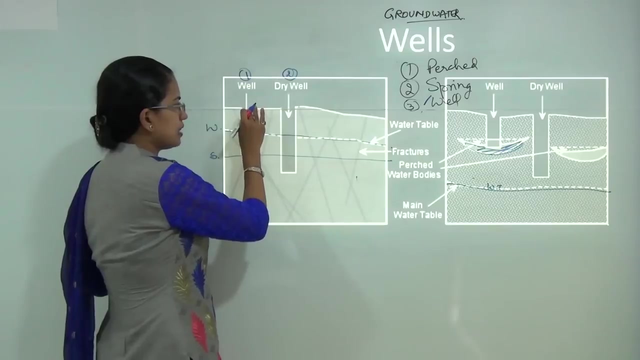 the water table. so water table say, this is the winter water table and this is the summer water table. two wells, one here, well 1 here and well 2 here, now during the winters as well as summers, what would happen? this well, which is the deeper well, would have water availability in both. 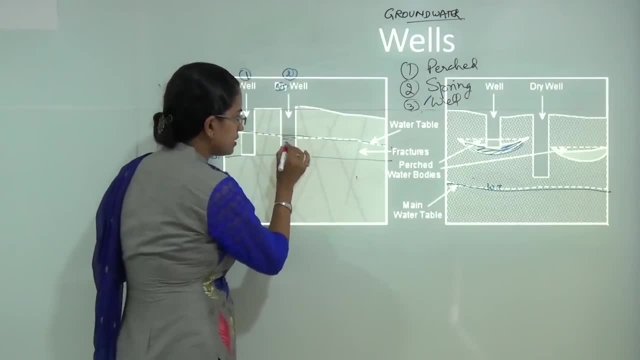 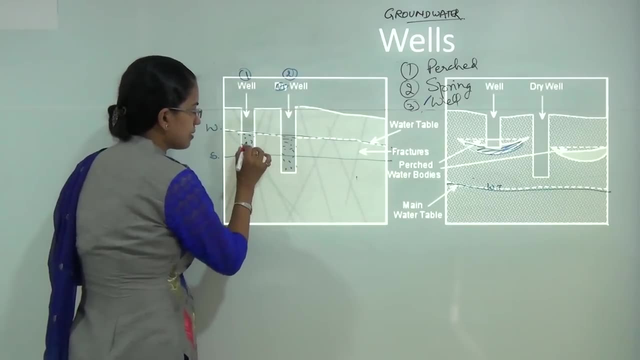 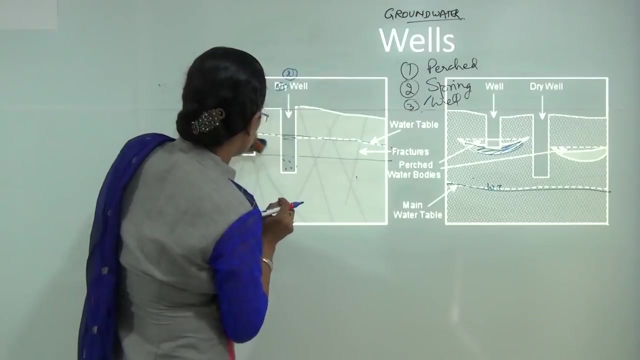 the cases, because the water table is still here, so water will be till here during the winter months. so this well would have ample of water again. this well would also have ample of water during the winters, but what would happen during the summers? during the summers, the water table drops down or the water level drops down. I could say, as a result, this new 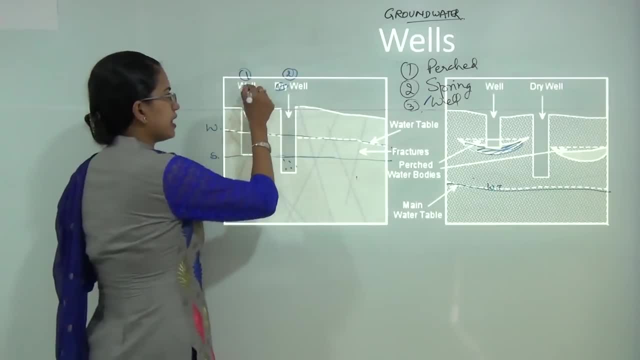 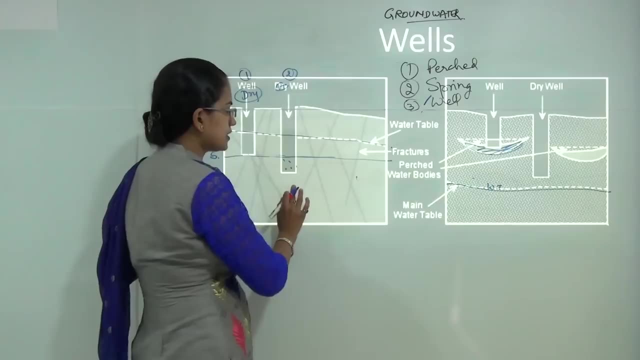 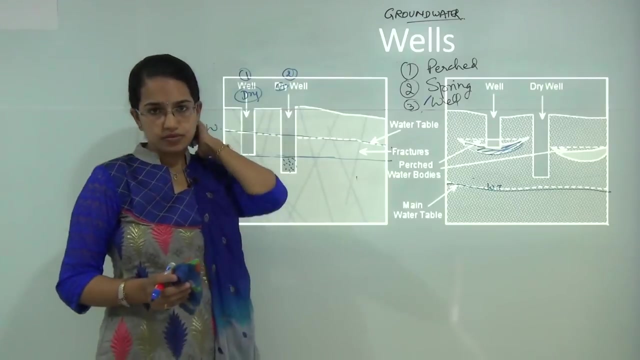 water table line is here. so what would happen? this well would dry out during the summers because there is no more availability of water here. however, well 2 would have ample water still, even during the dry months, because it is dug deeper. So this is how we understand the concept of well. now there are numerous factors that 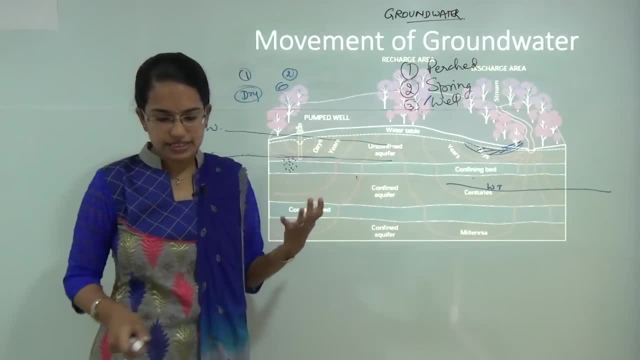 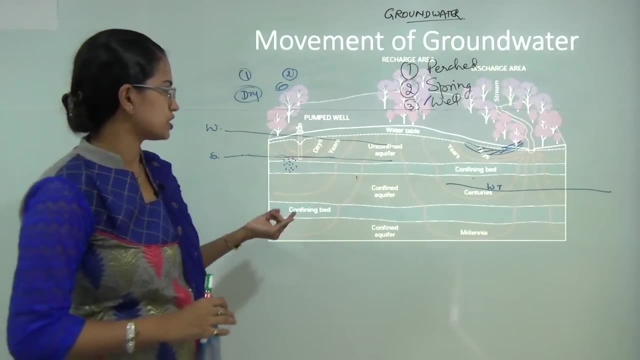 affect the movement of groundwater. when I say movement of groundwater, the movement can occur in the zone of aeration, the movement can occur in the zone of saturation. so let's talk about those one by one. when I say movement is occurring in the zone of aeration, it can. 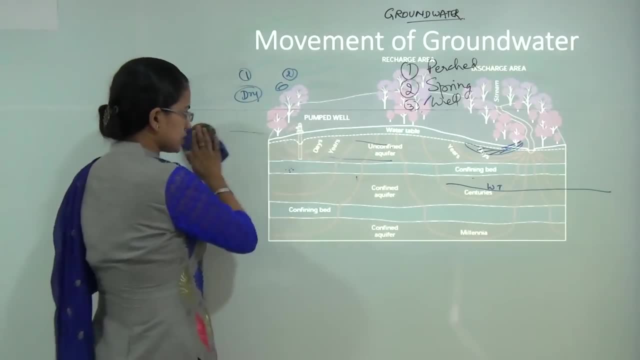 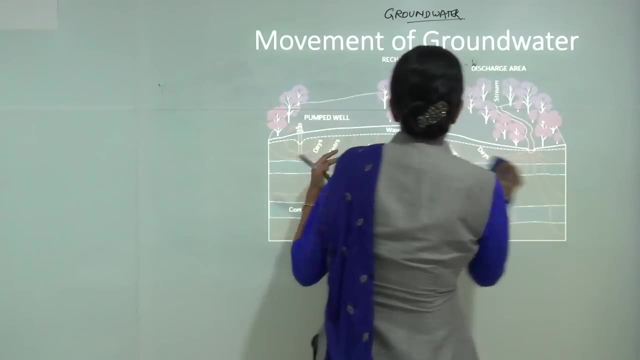 be due to numerous factor. it can be due to presence of soil moisture, it can be due to roots holding the water in that area. CLOSED CAPTION by Mrs Sibyl oui. region due to rainfall. so these are some of the basic reasons because of which you have. 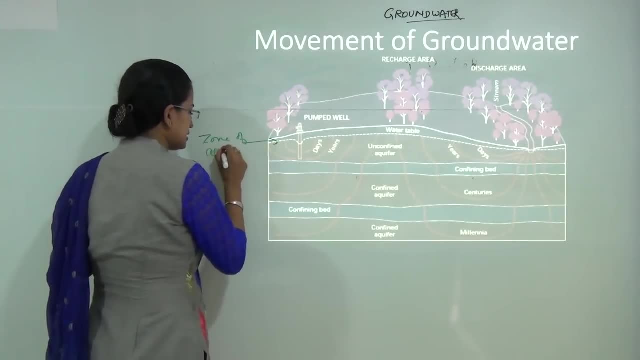 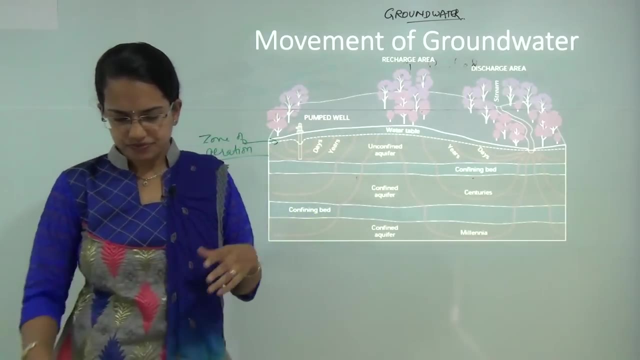 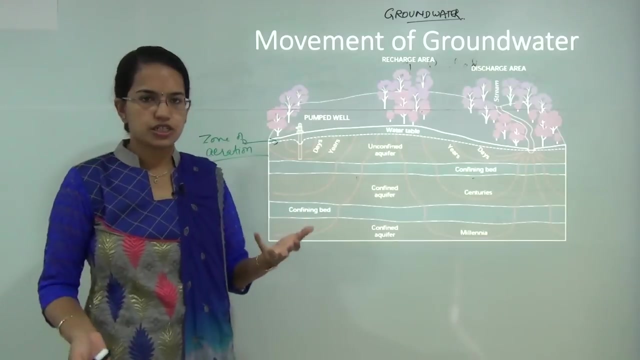 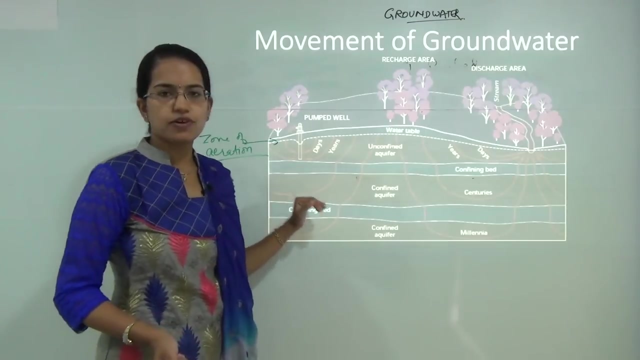 movement of water in zone of aeration, that's the unsaturated zone which is lying at a higher elevation. so you have absorption by roots, absorption by soil, absorption by plants, and then you have the natural rainfall that is occurring. all those would lead to movement of water within the zone of aeration. now what would be the case in zone of saturation, as 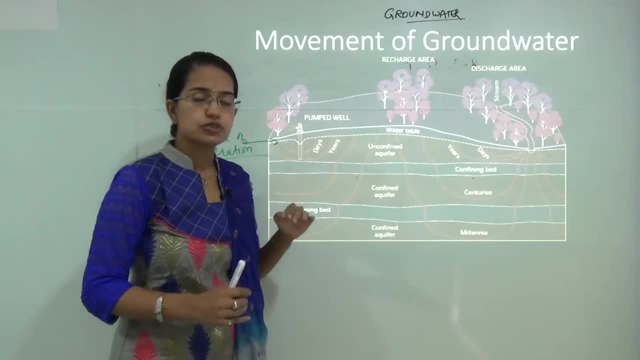 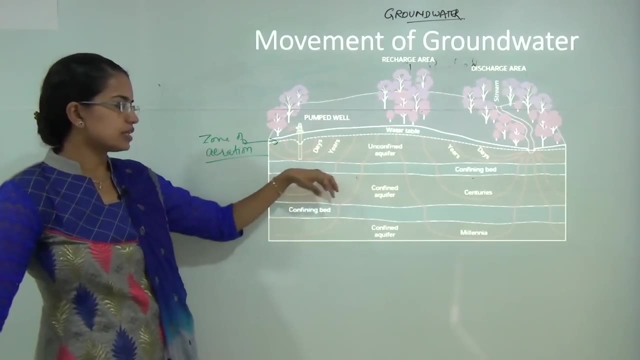 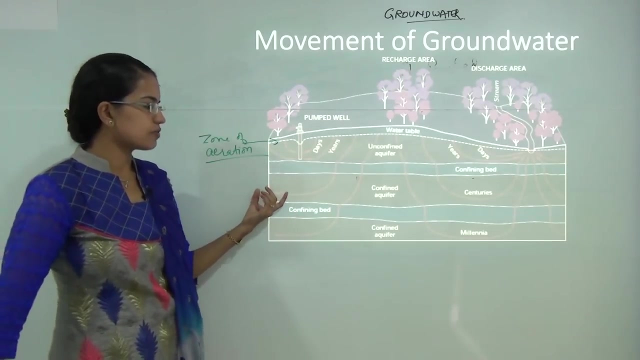 we saw it in the first demonstration: ground water moves, but at a very, very slow pace. so what would happen here? the water that is percolated within the interconnected pores would be present in the saturated zone and, as a result, in this zone it would be mainly gravitational force. 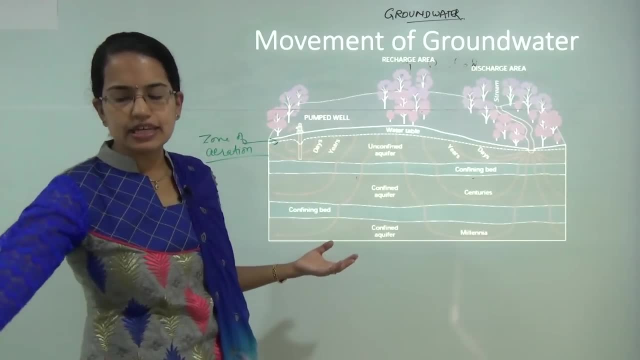 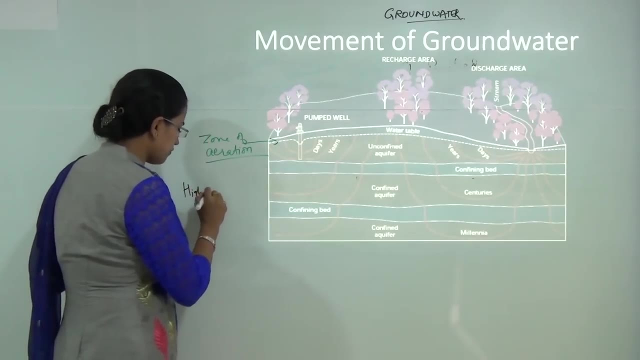 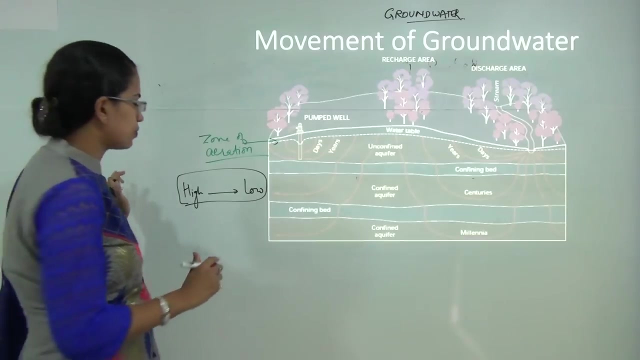 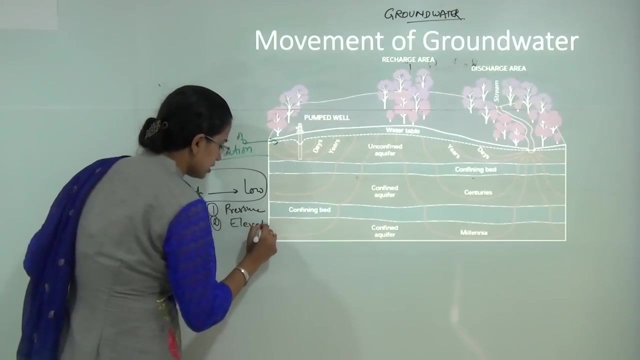 that would be responsible for movement of water. again, when I say movement of water there is, I could say. water tries to maintain equilibrium, so it moves from the region of higher pressure to low pressure, and the two main governing factors that promote the movement of ground water would be, first, the pressure conditions and second, the elevation. based on this there, 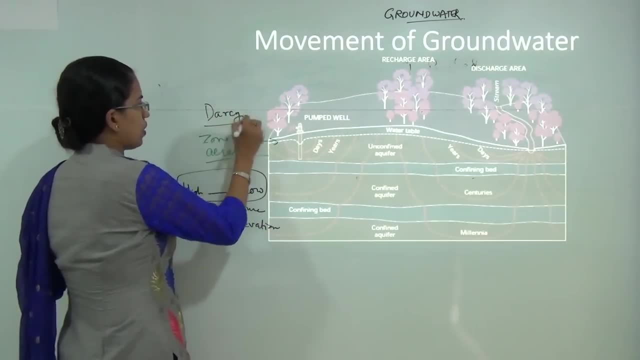 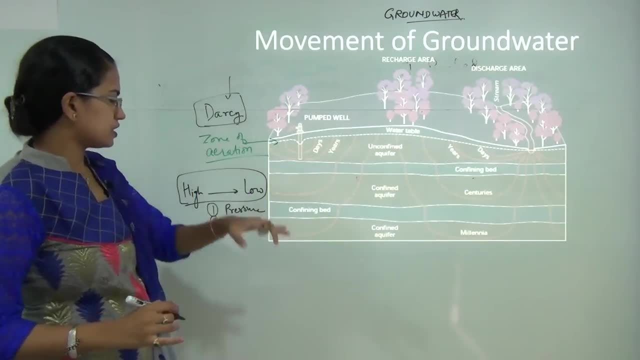 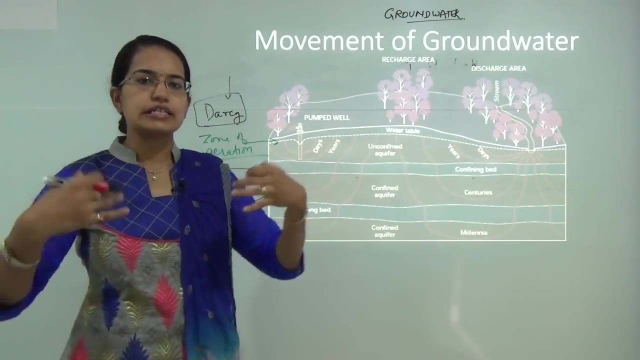 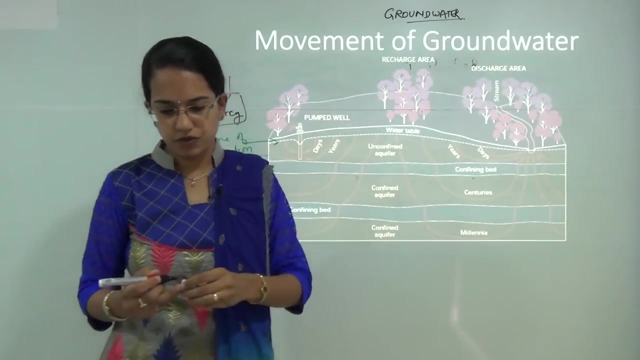 And Darcy is also known as father of hydrogen. Now we will be covering this further. now for now we try to understand the movement of ground water. so there is the concept of recharge and discharge. recharge means the water that is present here is recharged by the water that is coming from the above surface. so you 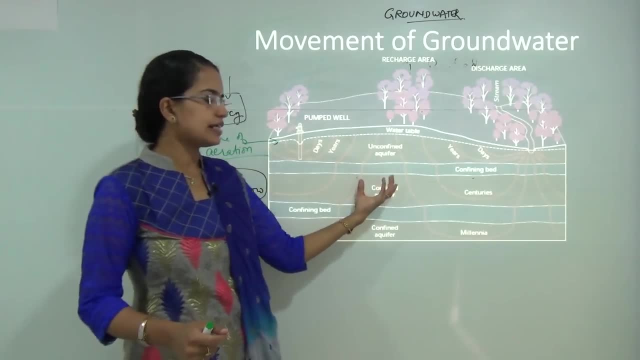 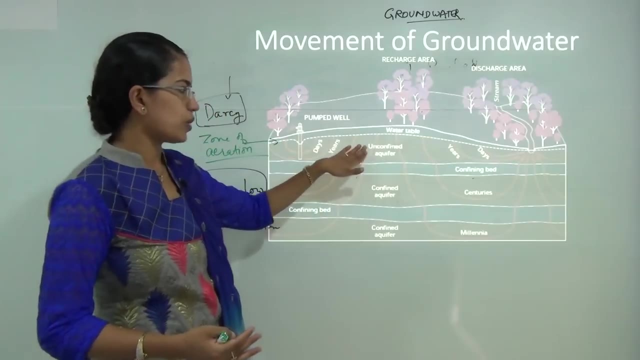 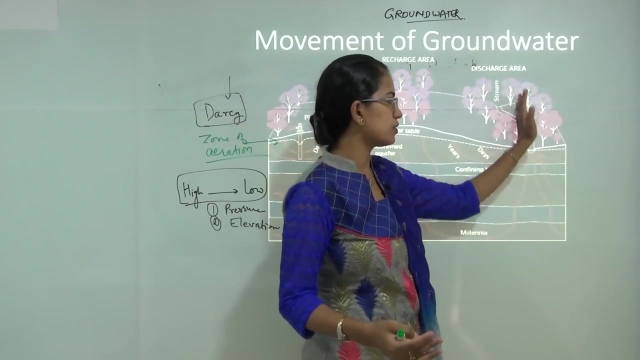 have the water that enters the zone, the saturated zone, and the saturated zone is further filled with the water means the water that is lying in the underground region moves to the main stream and it is being emptied out into the main stream, which is flowing here. 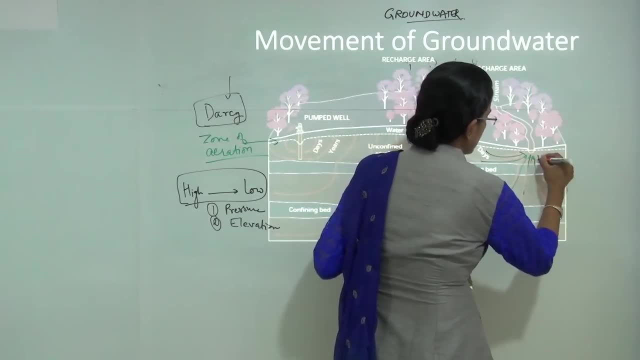 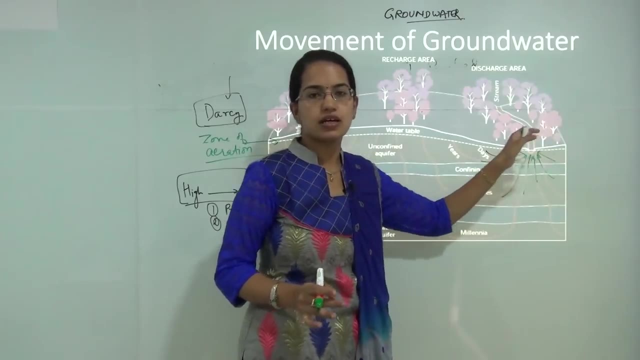 So this is where the discharge is taking place. If the recharge is greater than discharge, I can say there is ample of water. however, if the discharge is predominant as compared to recharge, there would be shortage of ground water table or I could say there can be dry zones. 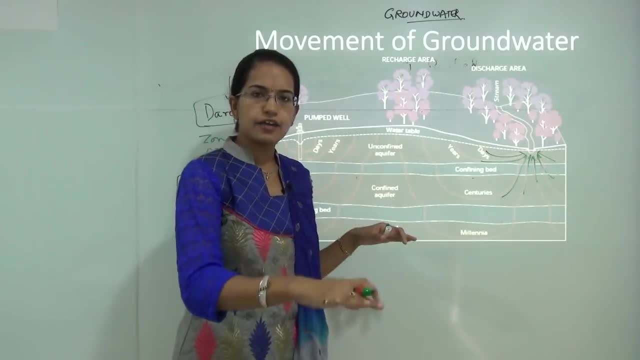 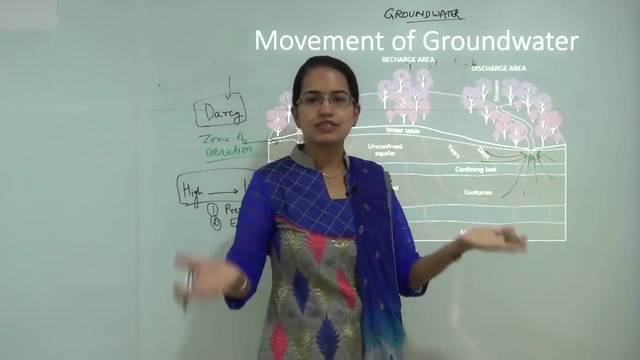 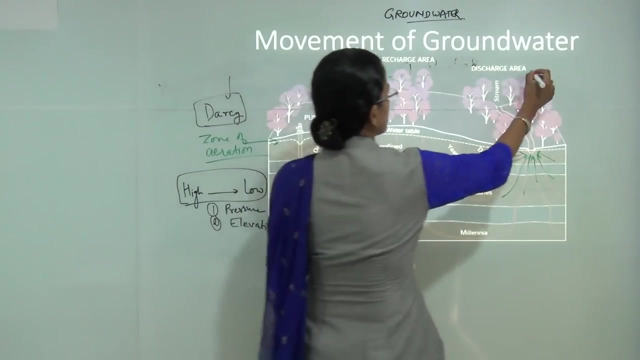 Dry zones is commonly used terminology to indicate drying or lowering down of the water table in most of the urban areas these days. So that is how we understand the balance between recharge and discharge. So recharge is filling up of the ground water, however, discharge is emptying out of the ground. 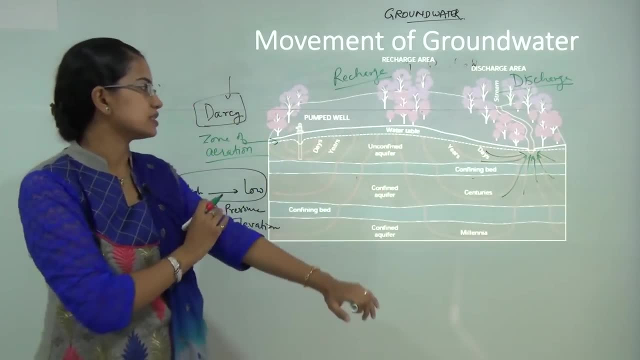 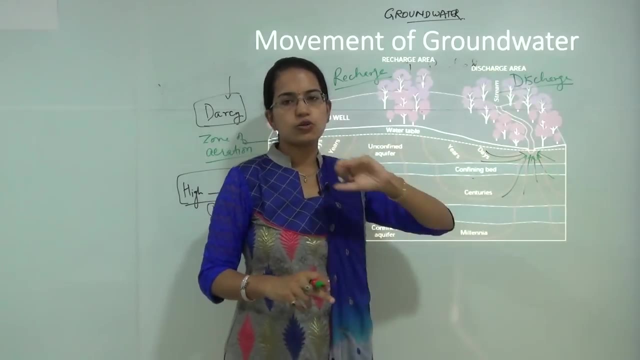 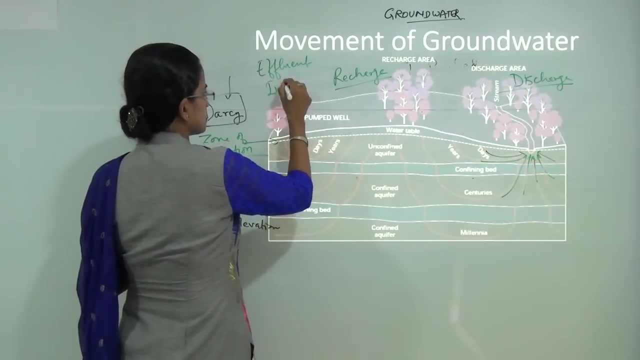 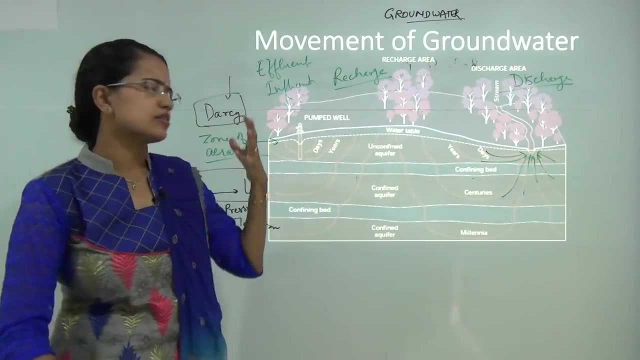 water into the nearby river or the main surface region. So this is the process that continuously takes place. However, besides these, there are two other mechanisms that we must focus on: the two streams: the effluent streams and the influent streams. Effluent streams are the streams or river bodies, rivers that feed. those are feed by 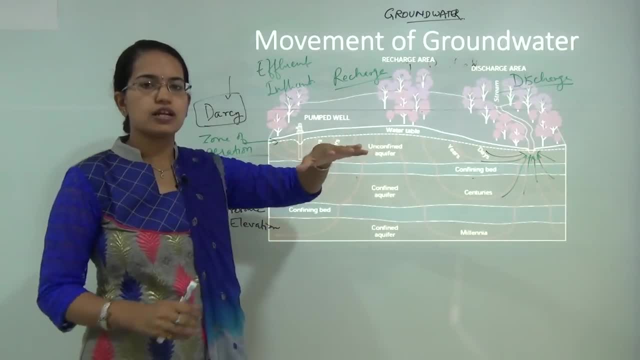 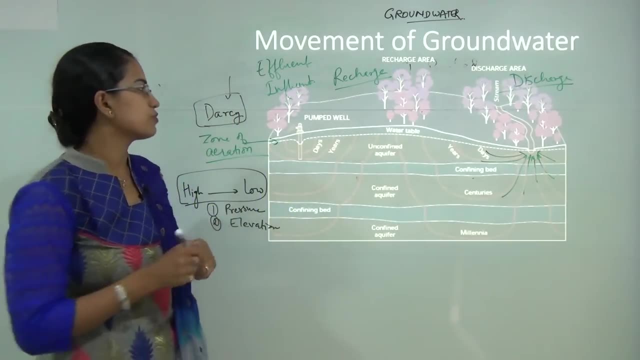 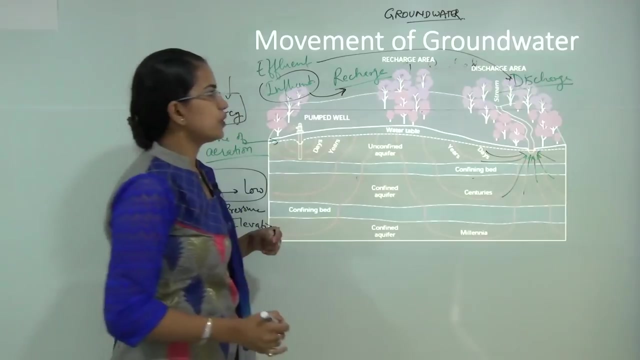 fed by the ground water. So basically, they are surface water which consumes the ground water. however, influent streams are those streams which contribute to the ground water. So these influent streams Lead to recharge and in simple terms I can say: and these effluent streams are predominantly- 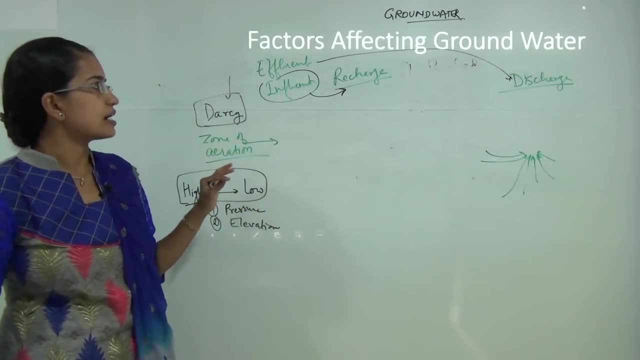 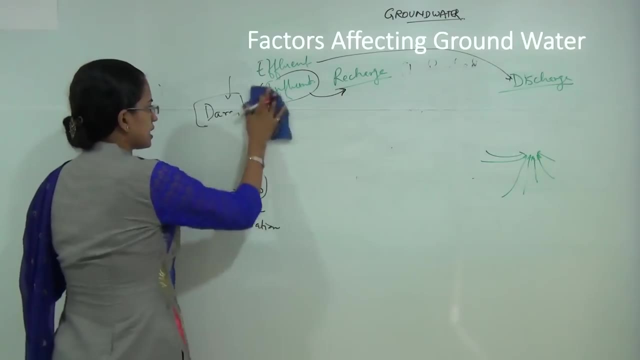 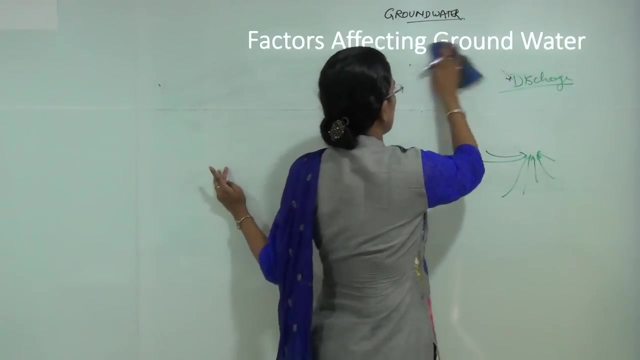 responsible for discharge. So this is how we understand the movement. now, when we talk about factors that affect groundwater, there can be three basic factors that can that we can understand for now. the first is the porosity, the second is the permeability and third- I can explain by means of Darcy's. 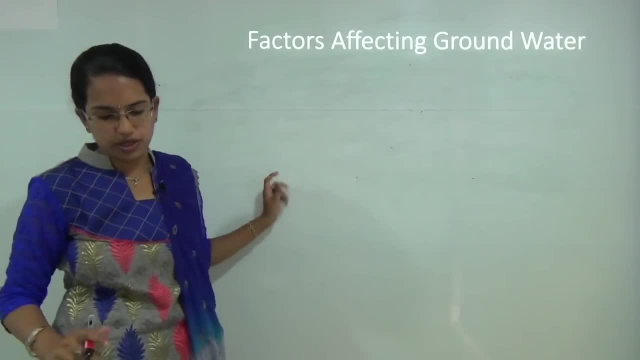 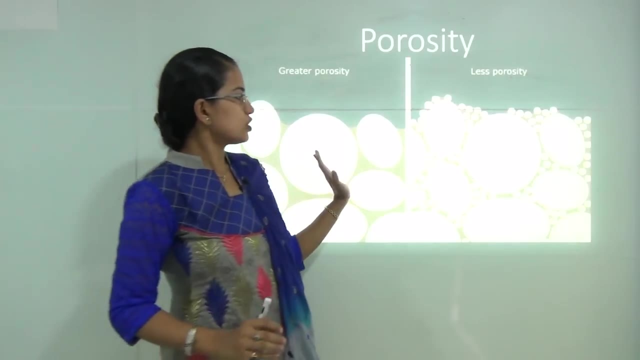 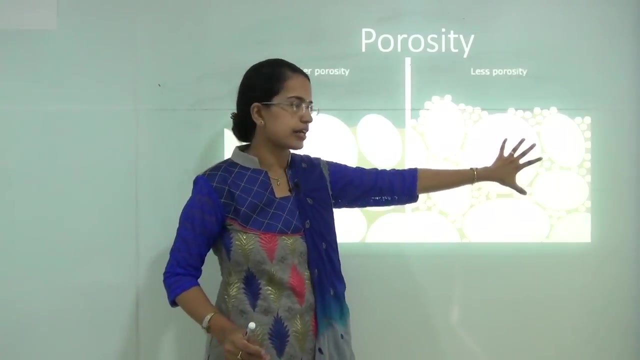 law. So when we talk about the factors affecting groundwater, we will discuss those one by one. the first is the porosity. So porosity, I can say you have two sections here, one towards your right and one towards the left. the one towards the right has numerous rock particles. 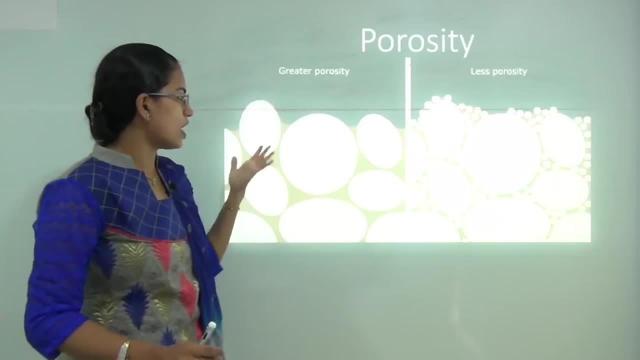 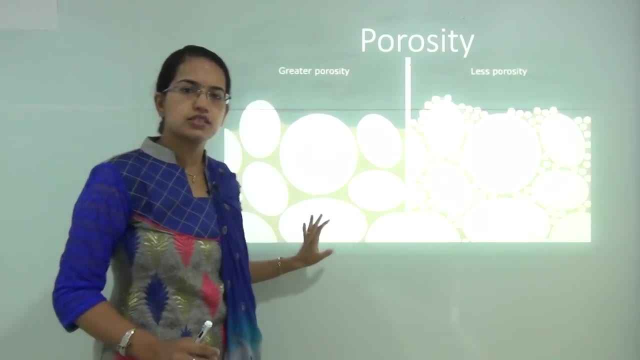 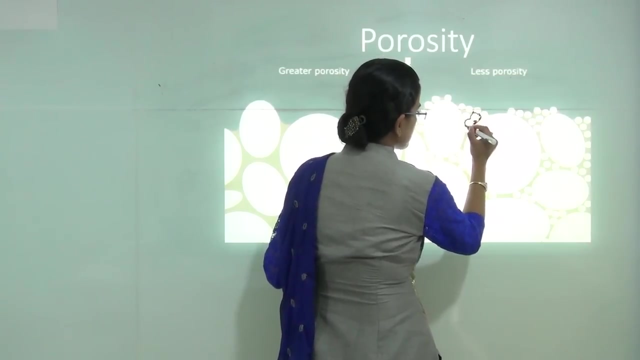 So you have bigger rocks as well as the smaller rocks. however, the one towards the left has just big boulders that are present. Now, what would happen? in either case, both of these rocks, I can say, are porous because there are empty spaces that can be seen between the boulders. however, the empty spaces here 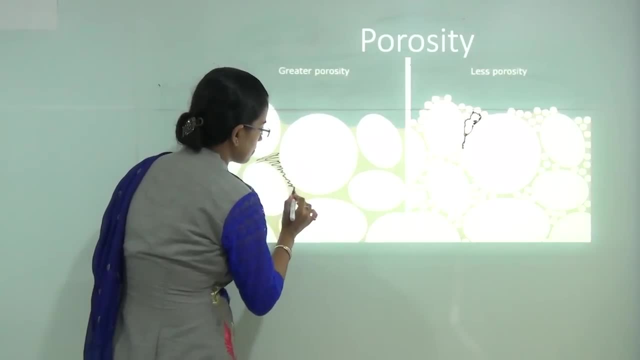 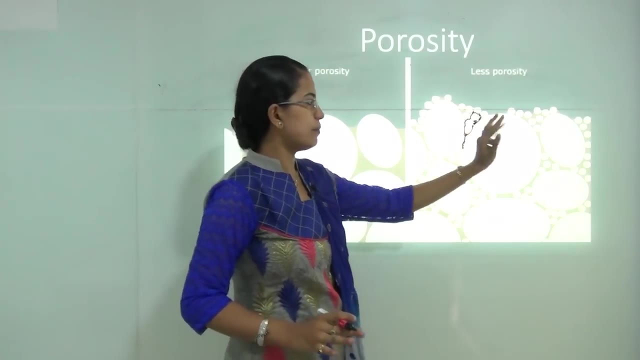 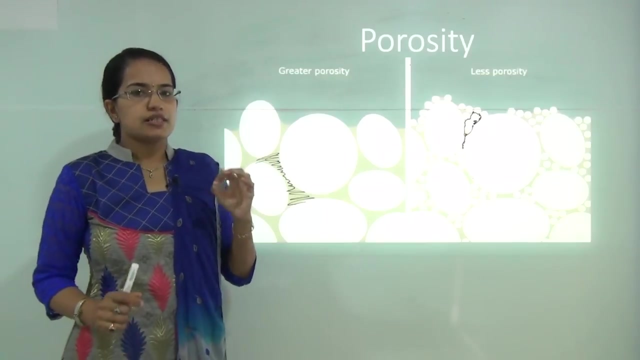 are much less as compared to the empty spaces that are present here. That means I can very simply say: this is more porous as compared to the one on the right. So that is how we try to understand porosity. porosity is the percentage of the rock volume. that is, Having Open open space or has pores. now, if I talk about the rock structures, the porosity varies. So you have sedimentary rocks, metamorphic and igneous rocks. first of all, the porosity of sedimentary rocks would be higher as compared to metamorphic and igneous rocks, because these 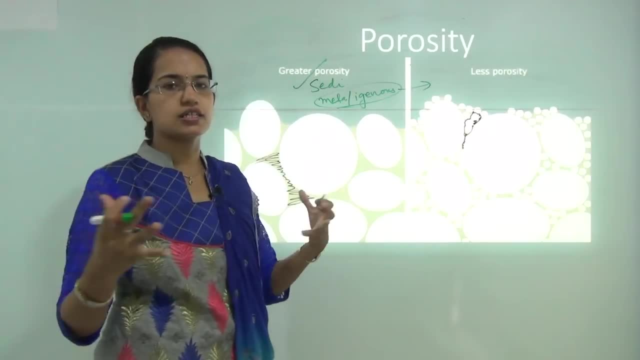 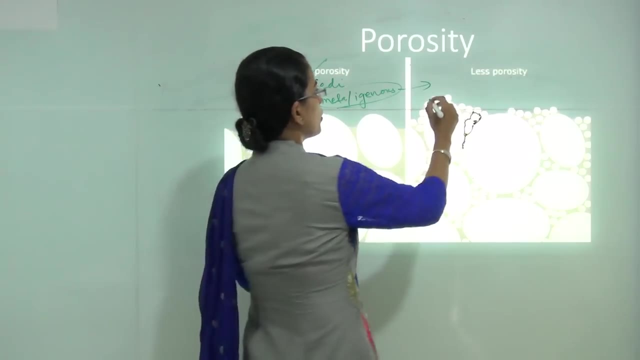 rocks are formed under high pressure and temperature, so there is more kind of compact rock as compared to sedimentary rocks. so these rocks are more compact and dense. as a result, the porosity would be less. When I talk about sedimentary rocks, I can classify these further into three types. 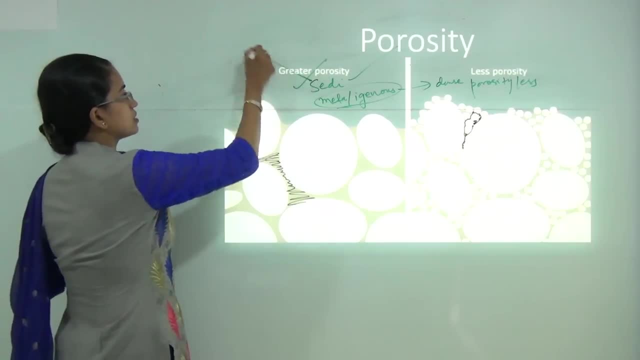 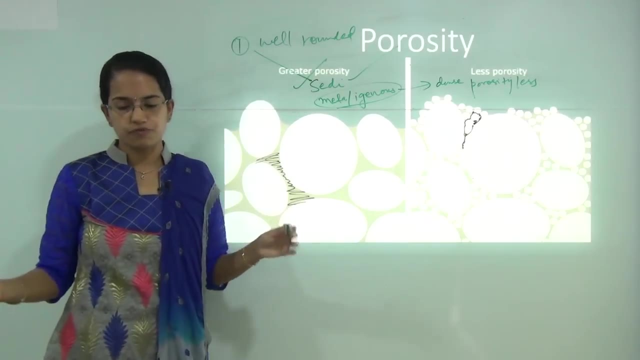 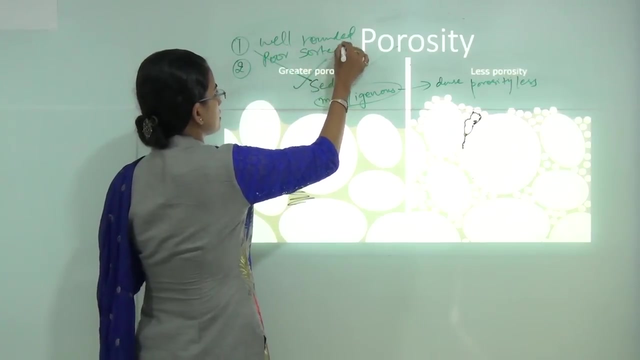 So one is a well rounded sedimentary rocks. A well rounded sedimentary rocks would have lots and lots of pores which are present within it. The second would be a poorly sorted rock. The second would be a poorly sorted rock. This poorly sorted sedimentary rock would have lesser amount of pores as compared to 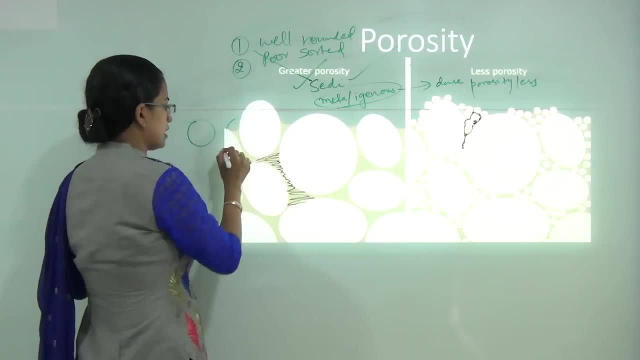 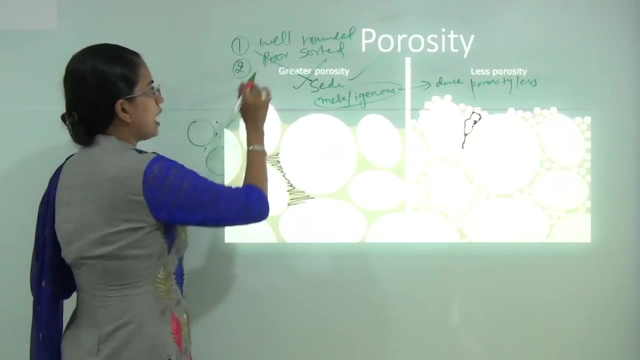 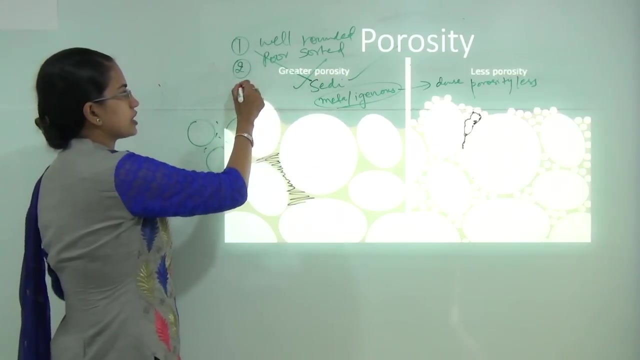 a well rounded, because one which is nicely rounded would be at a kind of equidistant position. so you have ample amount of pores that are present. however, one which is poorly sorted would have comparatively lesser pores than the well sorted, and finally you have a kind of highly cemented rock or which is present nicely. 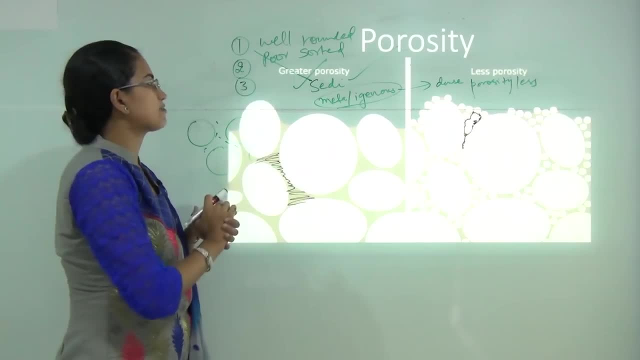 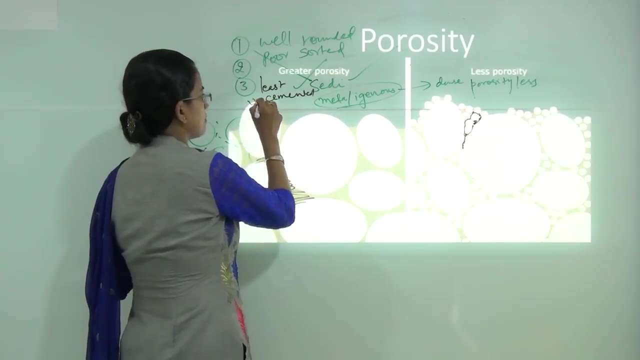 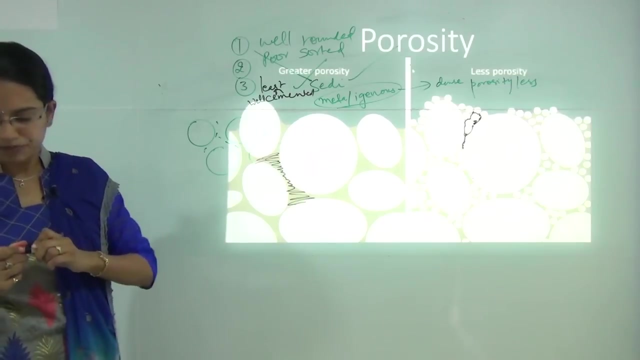 So this is a well rounded sedimentary rock. It is present nicely in a compact form and that would be least porous. So if I say well cemented rock, it would be least porous. So that is what is porosity. Now let's move on to the next concept, that is permeability. 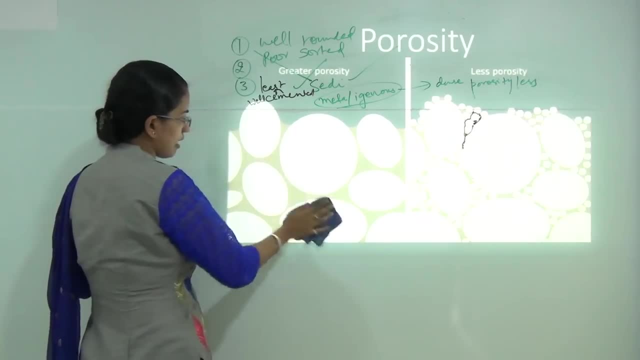 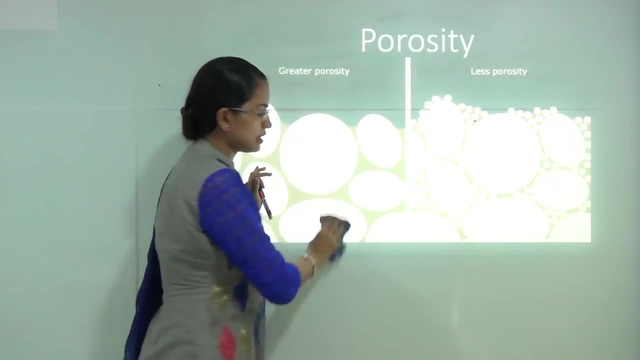 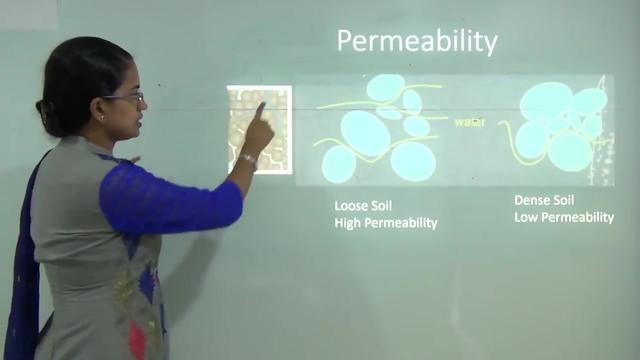 Now it's important the region with high porosity can have high permeability, and vice versa might not be true. let's see how. So let's understand what is permeability. Permeability, as I said, is the flow of liquid. as you can see, the liquid is flowing here. 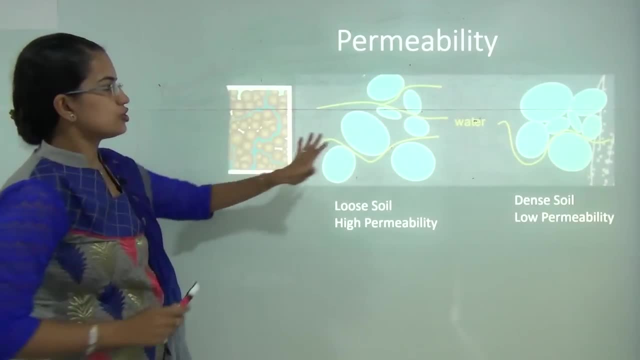 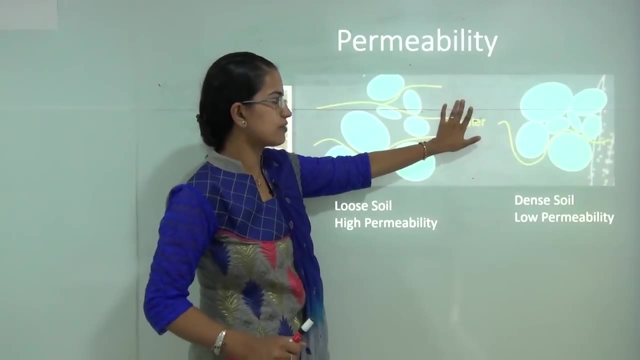 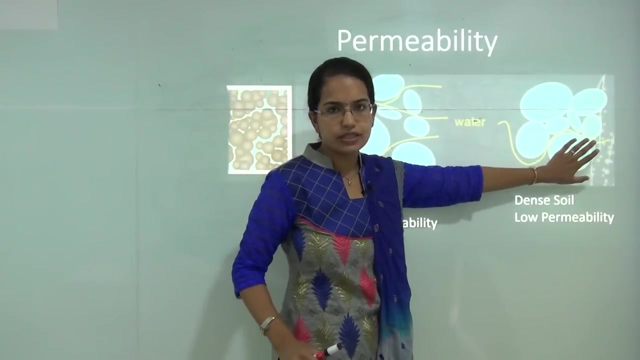 so it's the amount of liquid that can flow through the region. So you have the two sections of the rocks that are present here. this section allows ample flow of water or liquid. however, this soil section does not allow ample flow of liquid. that means this soil is much more denser as compared to this soil and the soil which 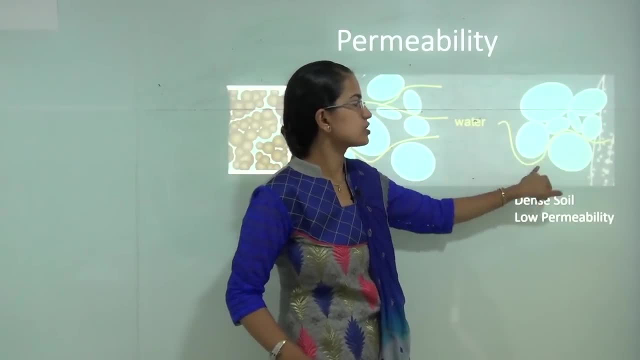 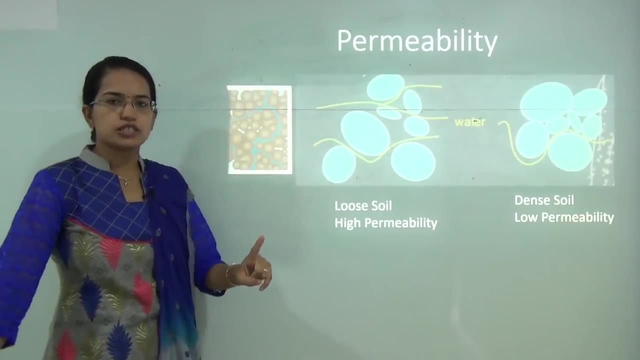 is more denser, So water flow is coming from the top of the soil and it's going to be less permeable because it's not allowing a smooth flow of water from within the region. So I can say low porosity means definitely low permeability because there is less pore. 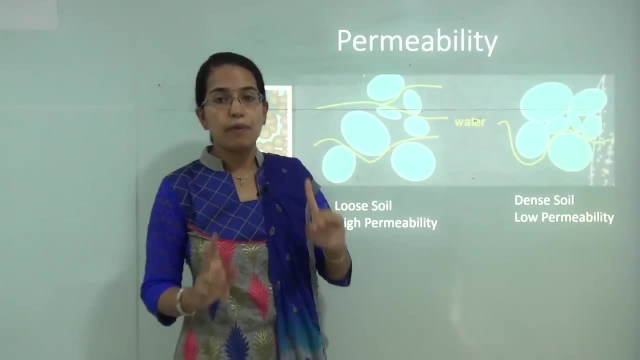 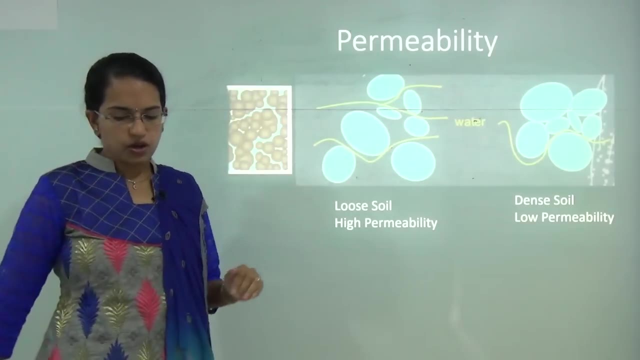 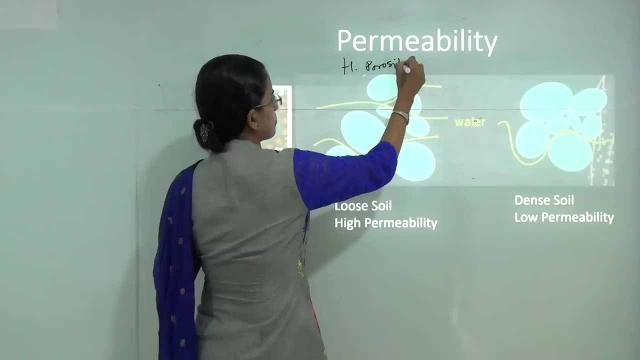 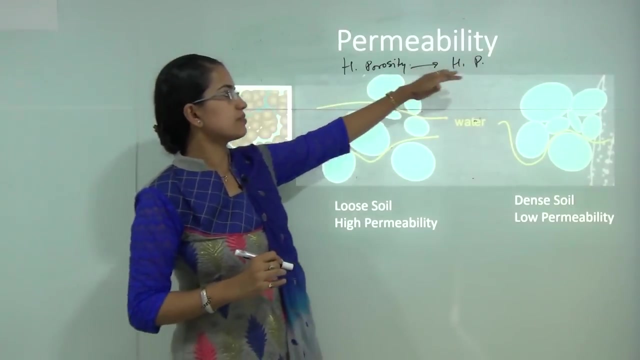 space. so movement of water would be less, that's for sure. but a region of high porosity might also have a low permeability because there is less interconnected pores. So if I say high porosity, High porosity, High porosity, It might lead to high permeability. that is correct. however, if I say low porosity, it might 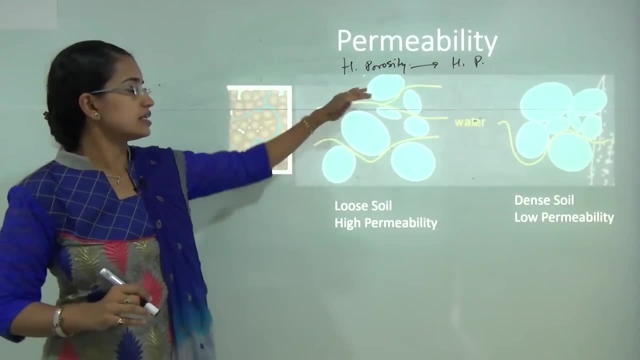 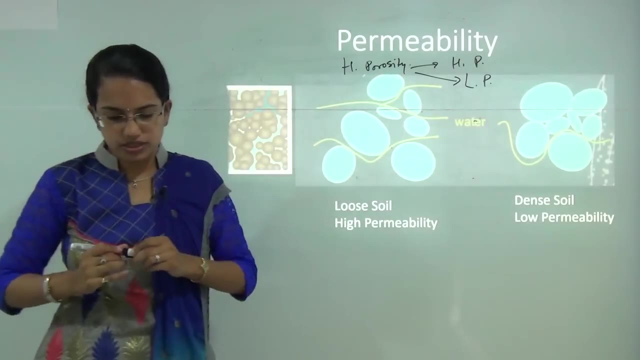 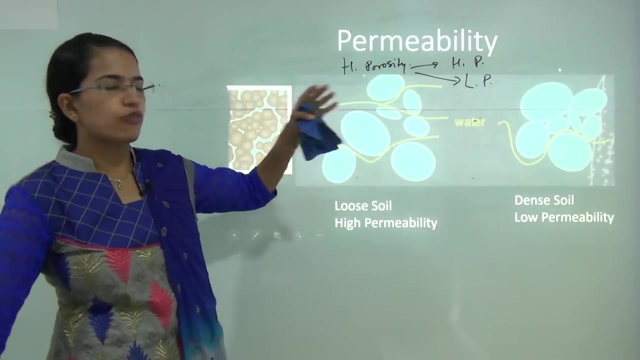 lead to low permeability, but there can be reasons where you have high porosity and it might lead to low permeability. the reason was. the reason, basically, is that rocks are not connected properly and, as a result, the flow of water is not smooth. so, as a result, 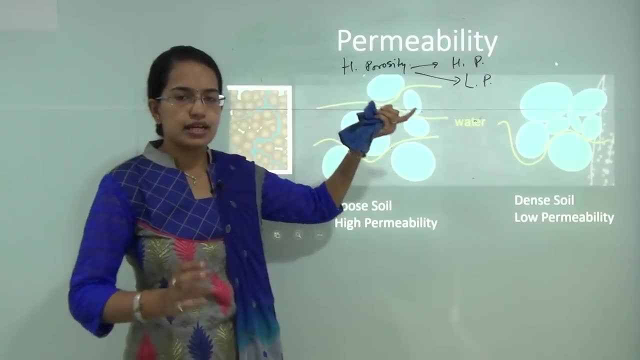 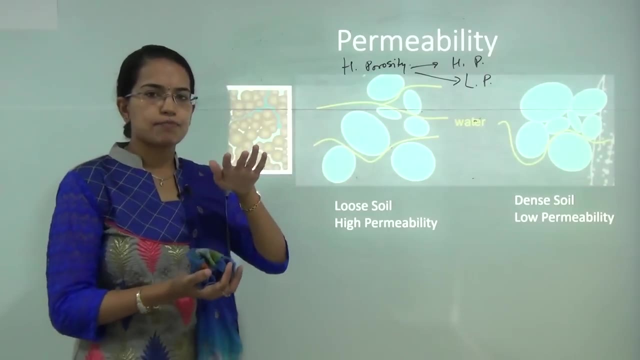 there would be lesser permeability. a good example can be clay. clay, compared to other rocks I can say, has good porosity, but still, since they are compactly packed and there is less interconnections, it would have low permeability. so that is why we understand. 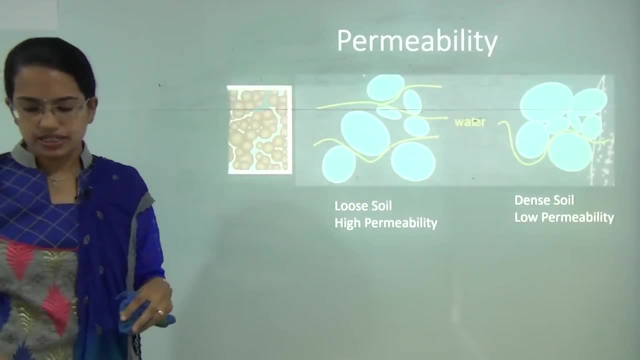 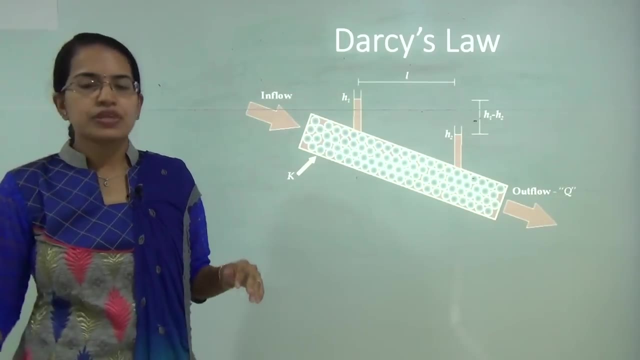 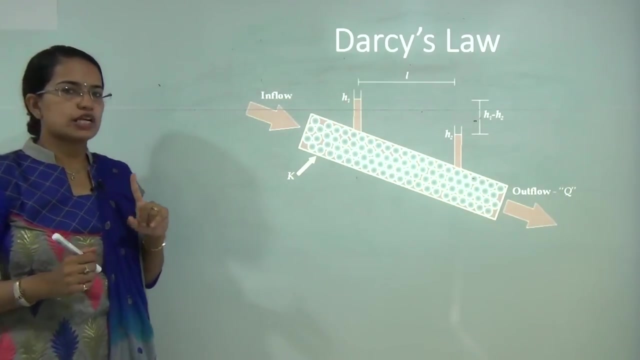 the concept of permeability. Now the final concept that affects the movement of groundwater is explained by Darcy, and that is known as Darcy's law. he said that movement is governed by two things: One is the flow of water, One is velocity and another is discharge. now, velocity first of all depends on the type. 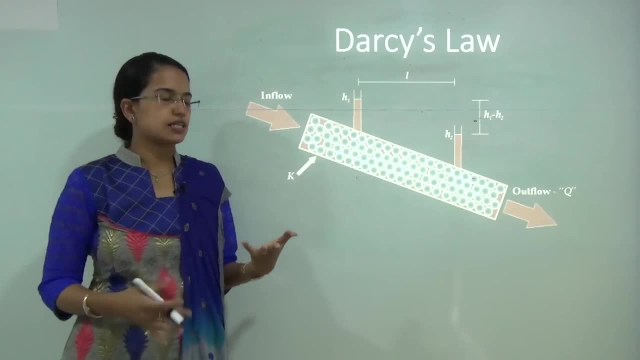 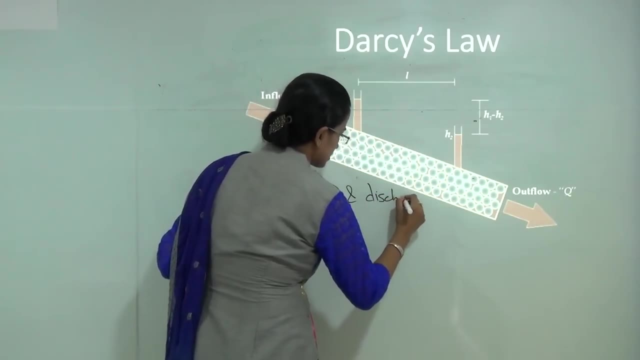 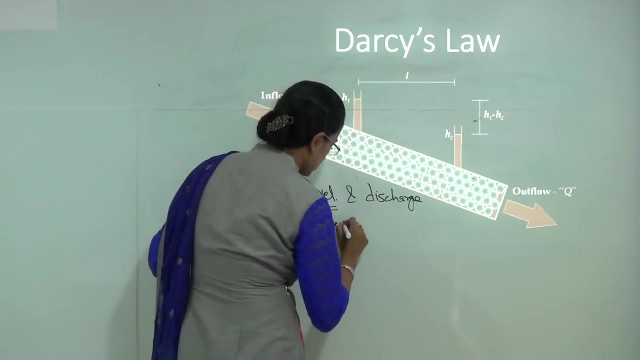 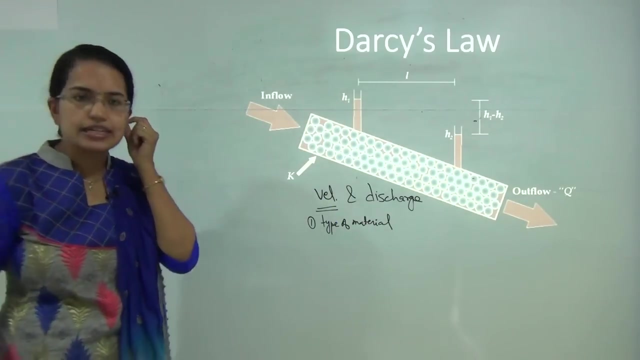 of material, so type of the fluid that is present would govern the velocity. so velocity and discharge was something that Darcy explained and he said that velocity is firstly governed by the type of material or its dependent on the material through which the liquid is flowing, and finally the hydraulic gradient, and he explained hydraulic gradient as the difference. 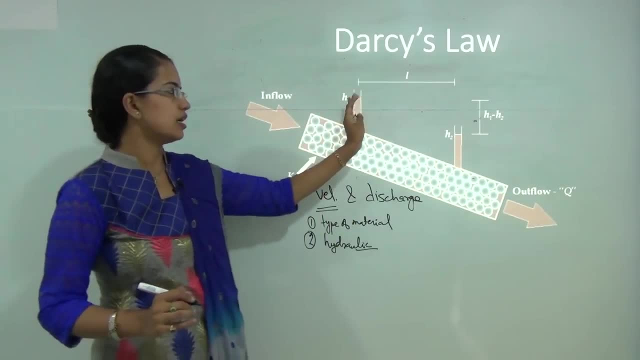 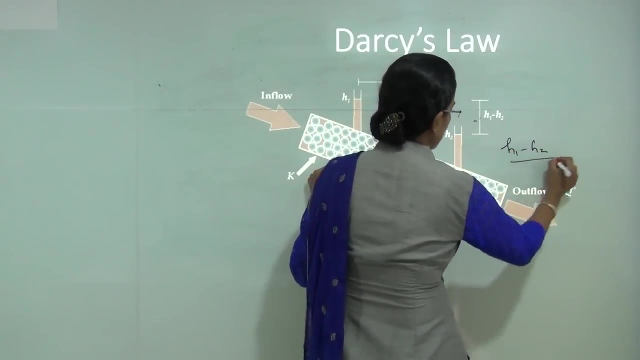 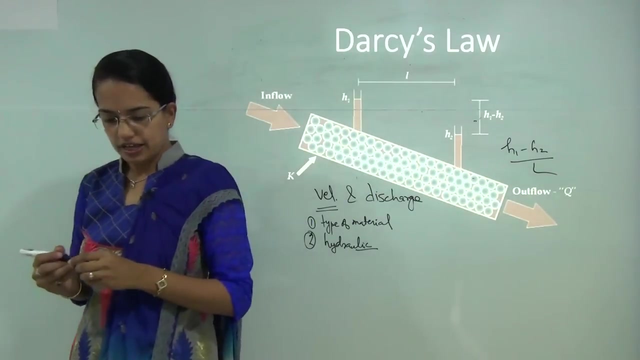 between the height and the ratio of the difference between the heights and the distance between the two. So he said so H1-H2 divided by the distance between two would be responsible for the hydraulic gradient. so higher hydraulic head would have more movement and higher connectivity, higher.